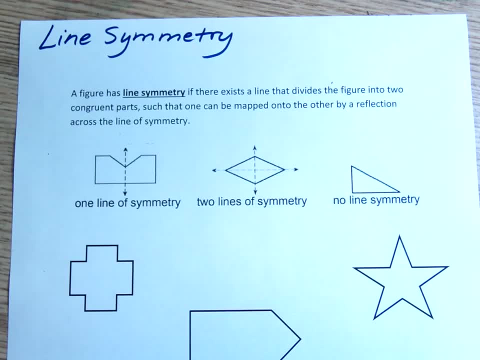 Hello Geometer friends, It's Ms Backfish, and I'm making this video for you to show you a little bit about line symmetry and rotational symmetry, two symmetries that are really important in geometry and actually in algebra as well, when we talk about functions that are even or odd, or neither really. 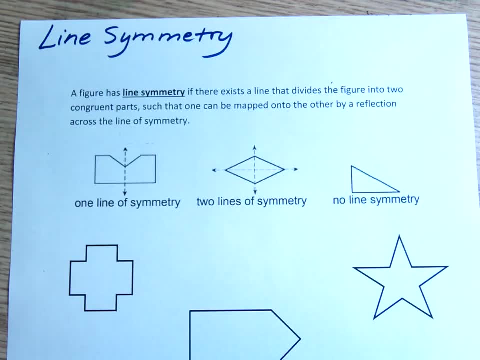 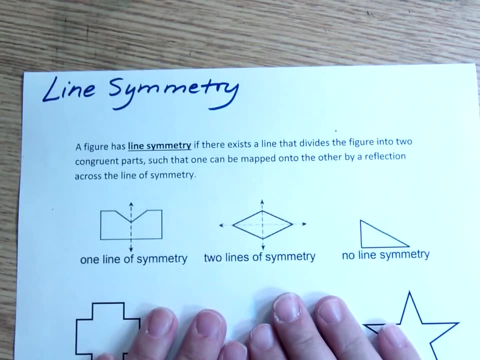 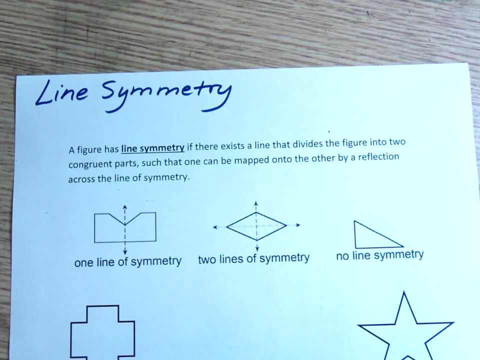 But specifically right now we're talking about line symmetry and rotational symmetry in the context of geometry. So I made this little worksheet thingy just to demonstrate and talk about it a little bit. But first of all, sort of defining it: A figure has line symmetry if there exists a line that divides the figure into two congruent parts. 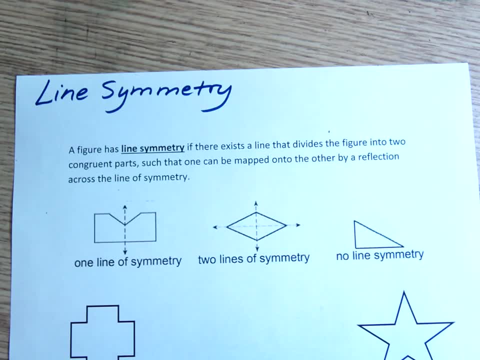 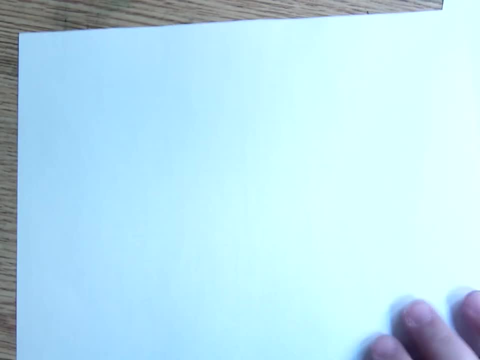 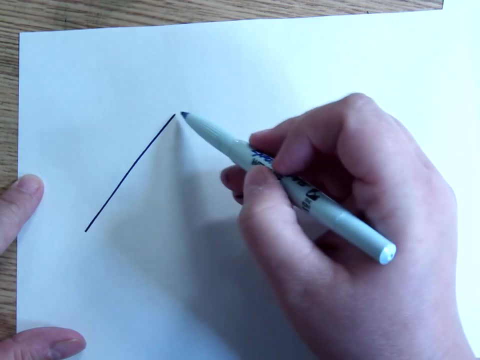 such that one can be mapped onto the other by a reflection across the line of symmetry. Now let me tell you why I added that part. Let's say, for instance, the last little phrase. Let's say: Let's say: I have 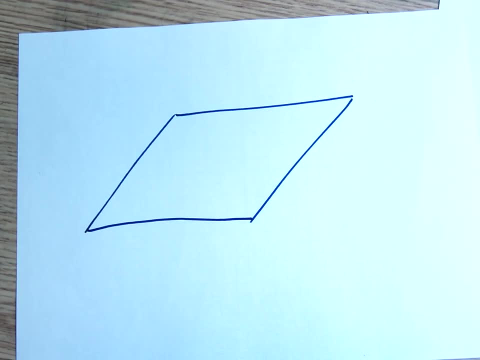 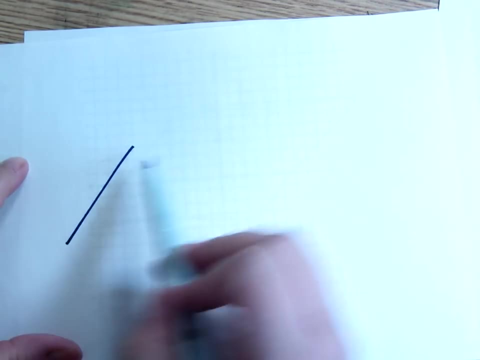 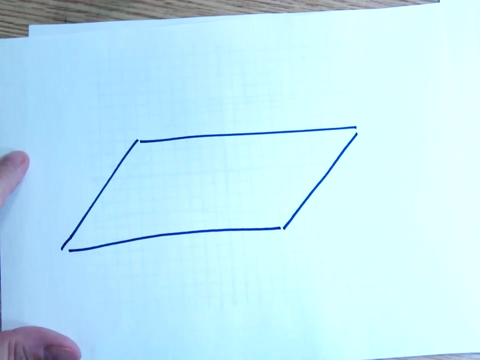 Let's not do this. actually, I'm going to draw a parallelogram, but I want to draw one a little bit more distinctly different in terms of the two directions, And I'm sorry it's lopsided, but that's really okay. 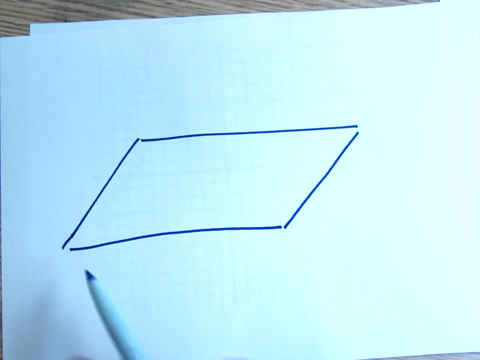 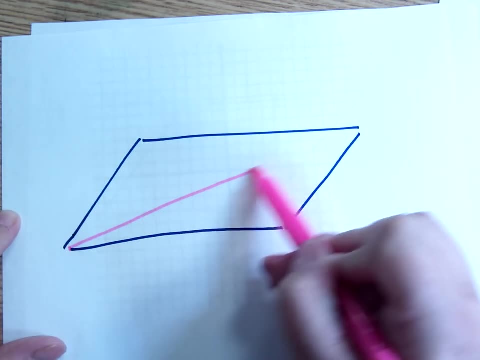 I'm not really worried that much about lopsided. If I were, If it weren't lopsided, if my parallelogram were more perfect and I drew a line right down the middle of it, then I would be dividing it into two congruent parts. 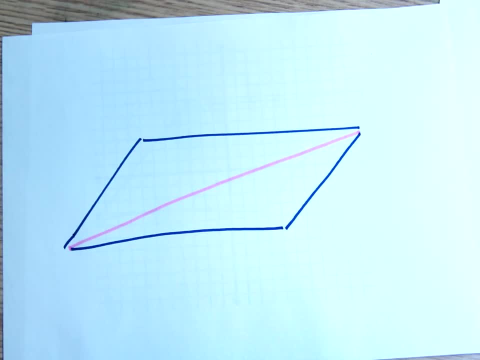 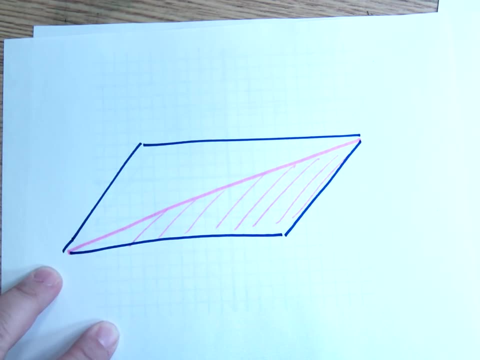 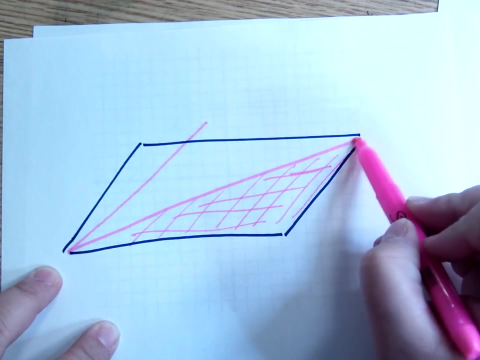 However, that's not a line of symmetry, Because if I take this side and reflect it across the line, Let me make that a little darker so you can see it a little better. It would be somewhere like this, Somewhere in here: 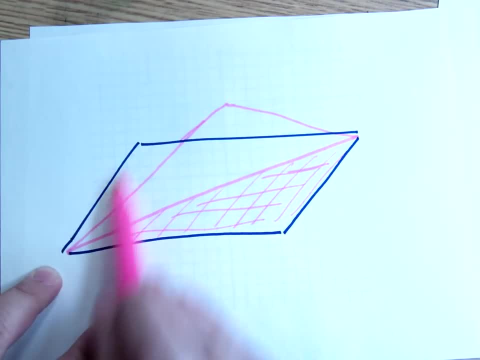 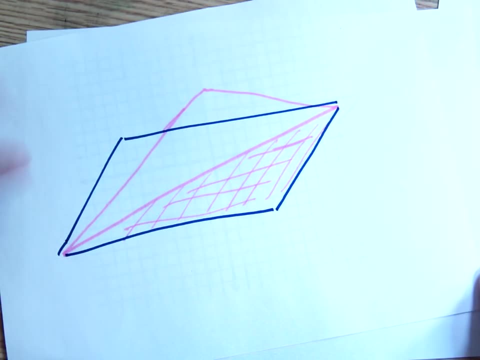 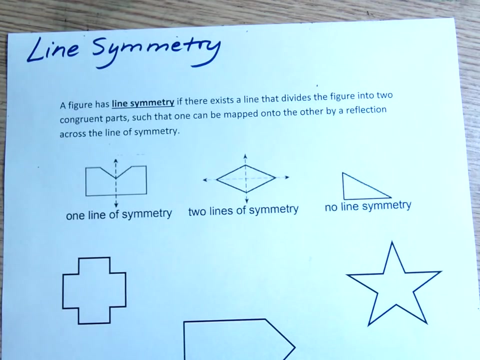 It would not be over there Where actually that triangle is. So you can have something. You can have a line that divides your figure into two congruent parts. that's not necessarily a line of symmetry or giving your figure line symmetry, So it specifically has to be so that basically, 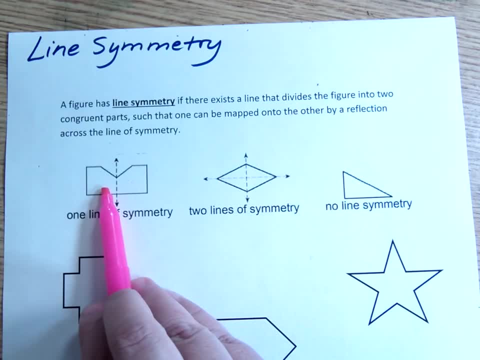 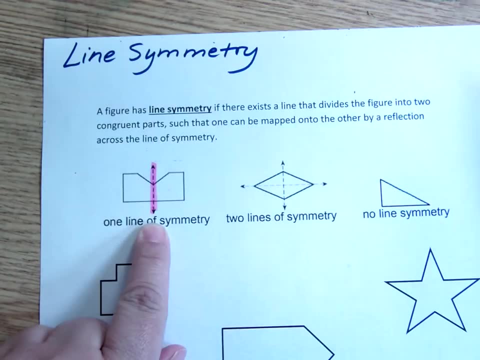 I can reflect one side over and it lands on top of the other side. So this figure right here has a line of symmetry right down the middle, The middle that's vertical here, Because these two parts here and here could be reflected. 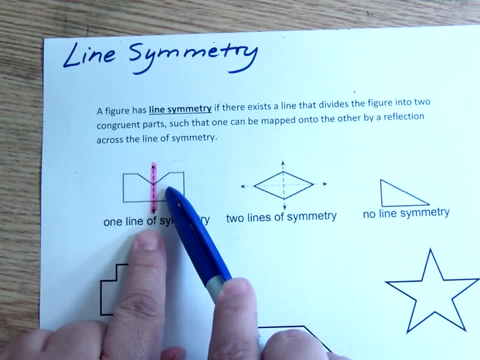 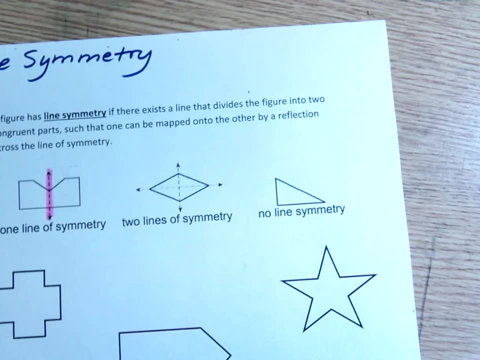 Either one of them could be reflected across that line and it lands right on top of the other one, meaning it maps onto it. Okay, same thing here, Except this time we have two lines of symmetry. We have a vertical line of symmetry. 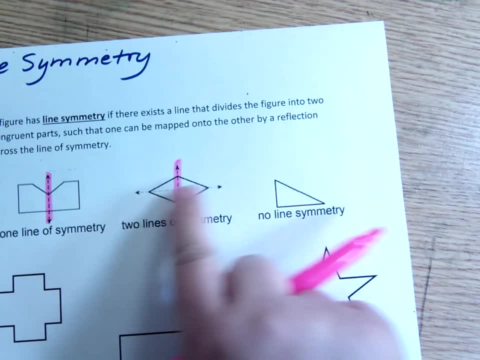 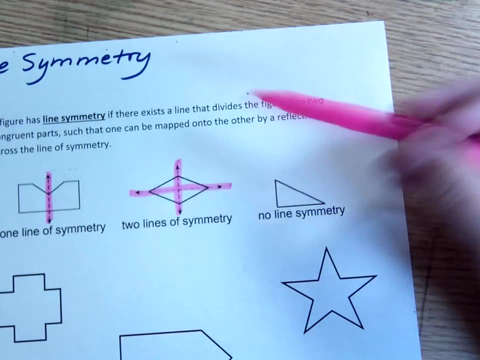 saying that I can reflect either of these two sides onto the other perfectly. Or we've also got a horizontal Line of symmetry saying that I could take the top of this and fold it down over the bottom and it would match up perfectly. 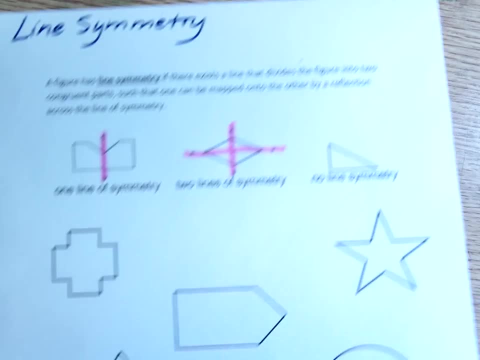 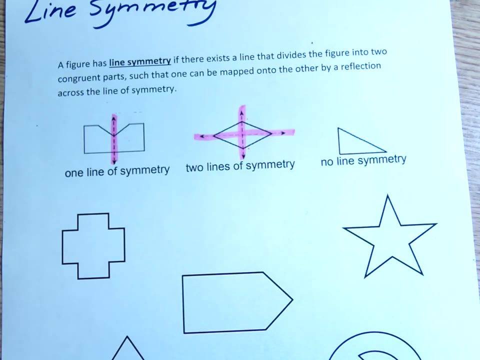 This one has no line symmetry. So line symmetry is really just the kind of symmetry- symmetrical- that you learned about in kindergarten. So if we have lines of symmetry, it's just the normal kind of symmetry you think of. So we have to figure out. 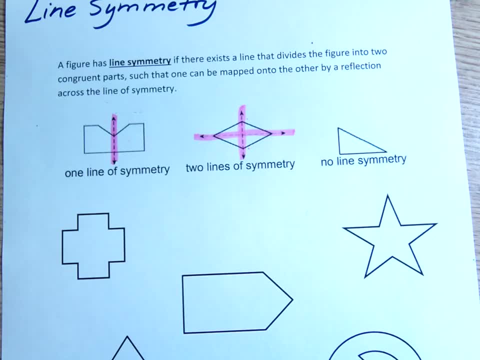 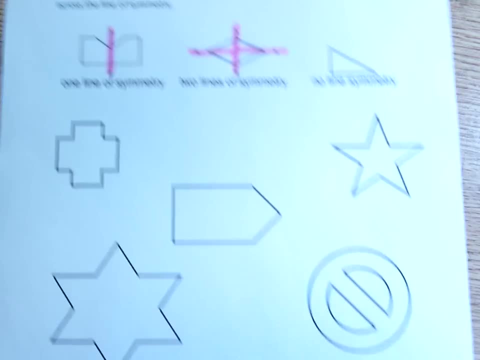 It's basically like you know, can I fold this figure into, Fold it in half on top of itself across this line? So these various figures I put down here were just some to look at the line symmetries of each one. 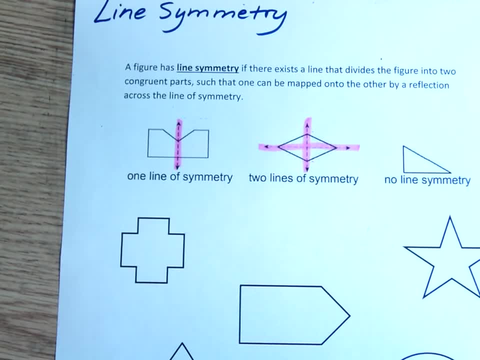 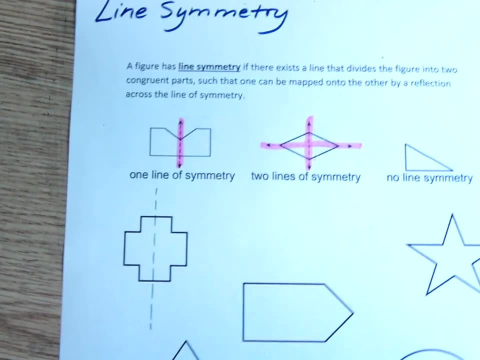 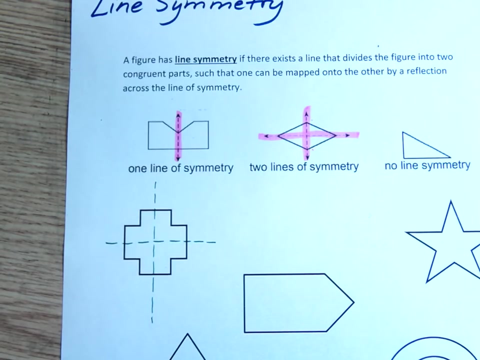 So this one right here looks a little bit like a red cross. I would say that it seems to have a line of symmetry vertically right down through the middle. I think it also has one horizontally right here. I'm also seeing two other lines of symmetry. 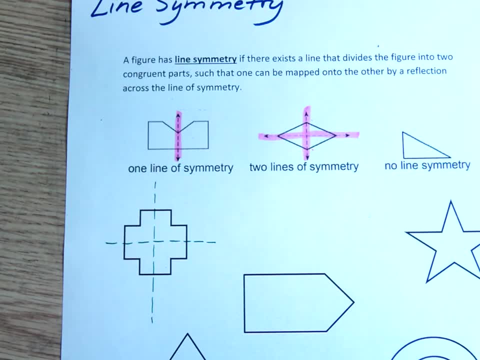 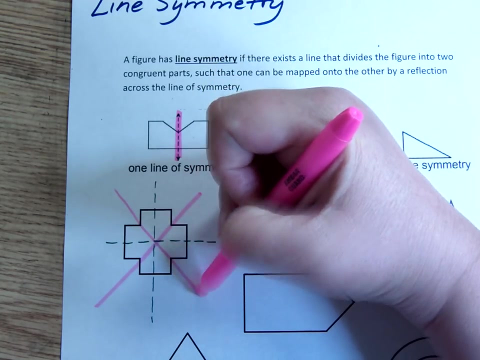 Let's see. Let's see if I can figure out what I'm thinking of. I would go ahead and say that there is also a line of symmetry that goes right here And another one that goes right here. So, basically, if I folded the figure over any of those lines, 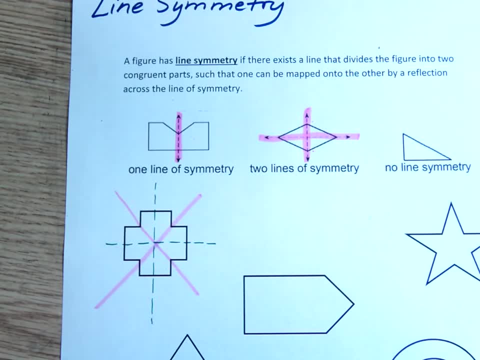 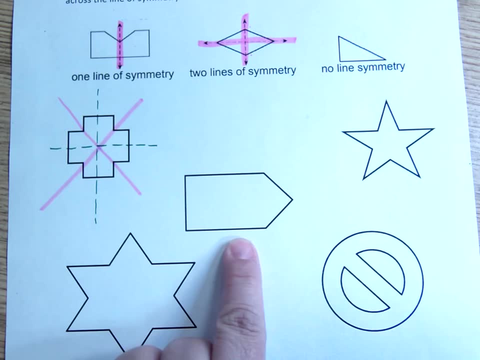 the two sides would meet perfectly. Okay, Now let's look at this figure in the middle Line, symmetry. Well, clearly, if I were to divide it right down the middle like this, vertically, that's not going to work Because we have a pointed side over here. 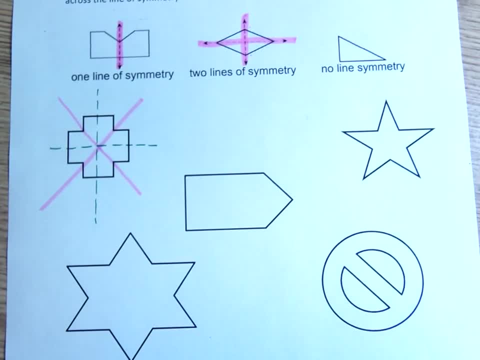 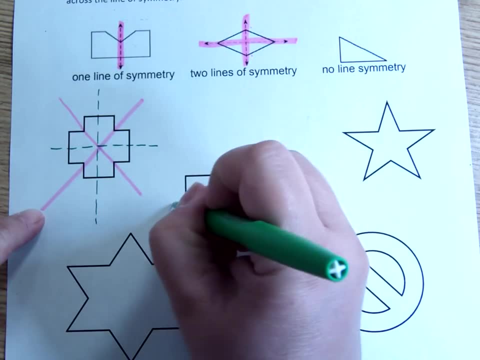 and it's not pointed over here. There's only one line of symmetry that I can see in this one. Where is it? You're right And I can hear you through this recording. Isn't that amazing? It's right there through the middle horizontally. 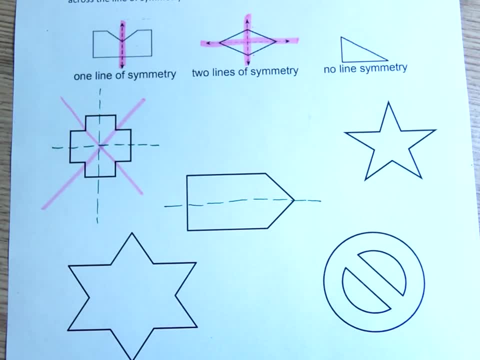 And much straighter than the one I drew. I actually got out one of my favorite straight edges to use for this and have been forgetting to use it, So I will try to use it on the next one- One of my favorite things to use as a straight edge. 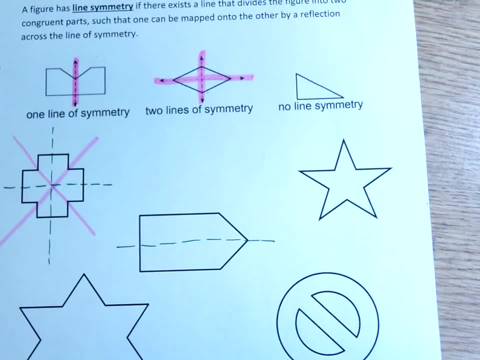 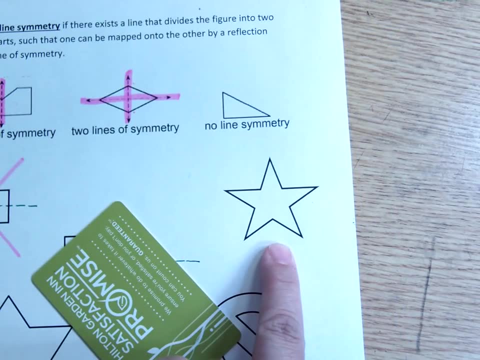 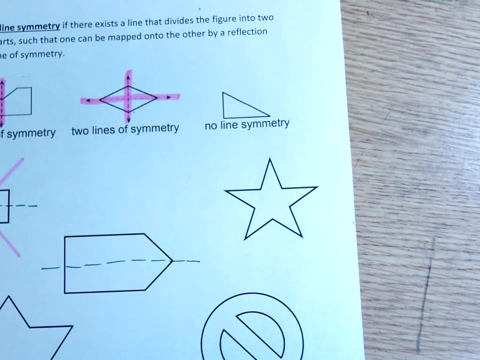 is an old gift card or hotel room key, They make a perfect straight edge. So, looking at this star right here, I'm going to use my perfect straight edge to make a line of symmetry or two, if I can find any. Okay, Think about whether you have any lines of symmetry in a star. 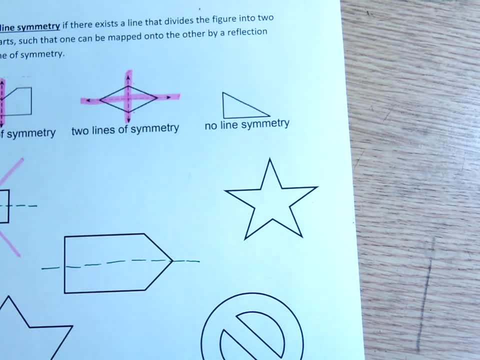 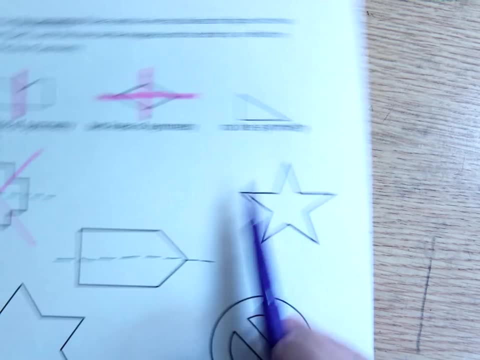 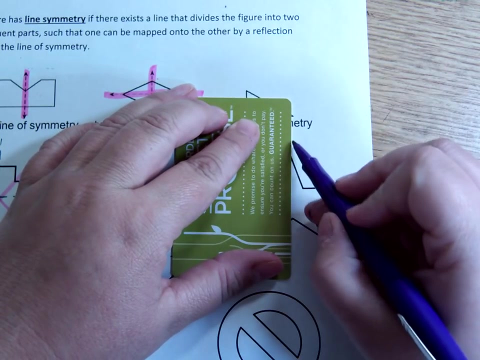 It helps on this one perhaps, to picture it as, like a person, Where this is a pointy head, two arms and two pointy toes. Well, right down the middle of a person there's a line of symmetry. So we've got a line of symmetry here. 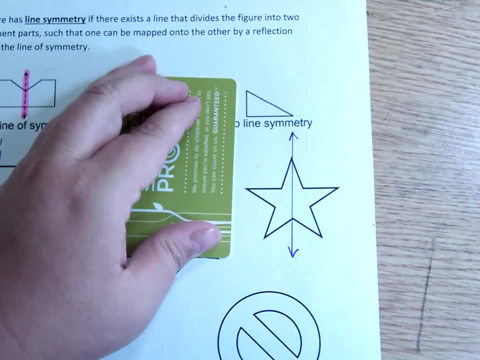 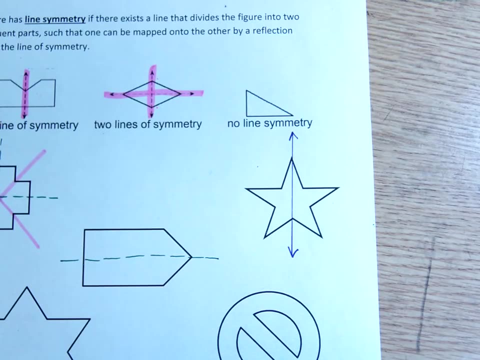 I'm not going to make it dotted, because it's a little bit easier to do this here. But then I can turn this star lots of directions and have a point at the top that I can think of as the head, The head of my person. 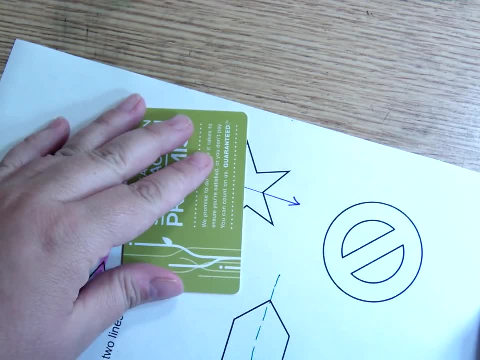 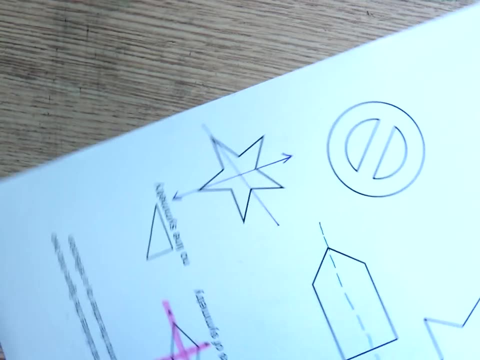 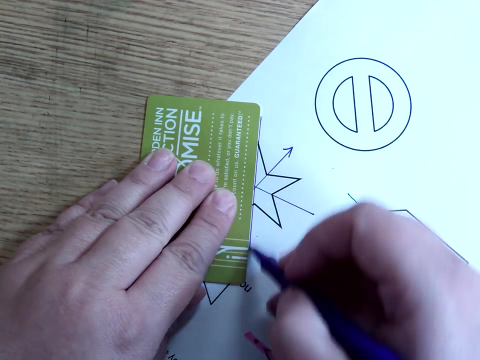 So, although it looks like it's not exactly symmetrical here- but that was me doing it with my clip art And that's my fault- We're going to pretend it is. So basically, there's a line of symmetry each one of these. 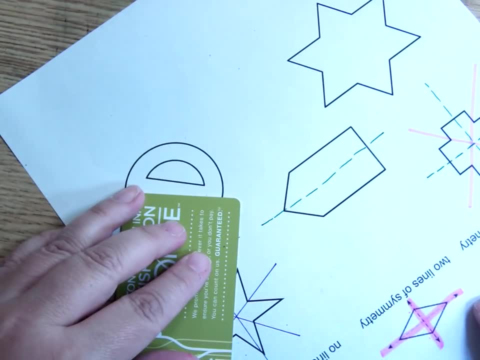 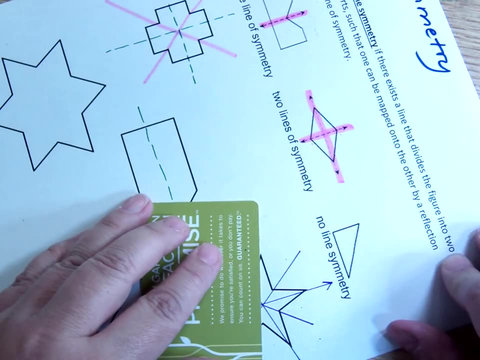 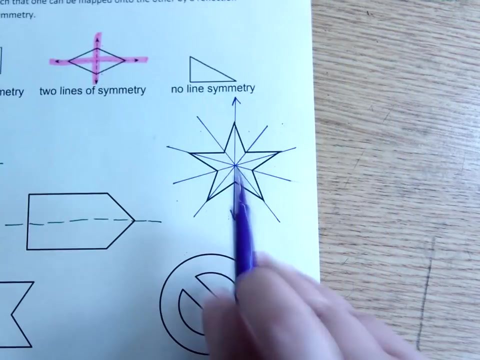 You could think of it as there's a line of symmetry that goes through each tip, each point of the star. So how many does that make? We have five lines of symmetry. We've got one, two, three, four, five. 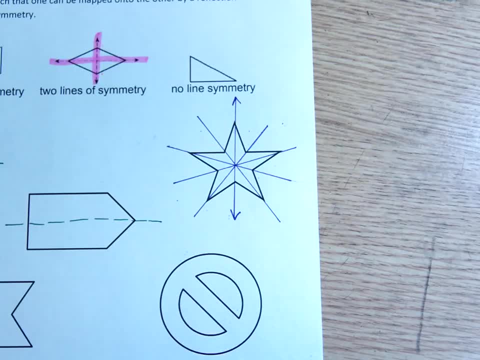 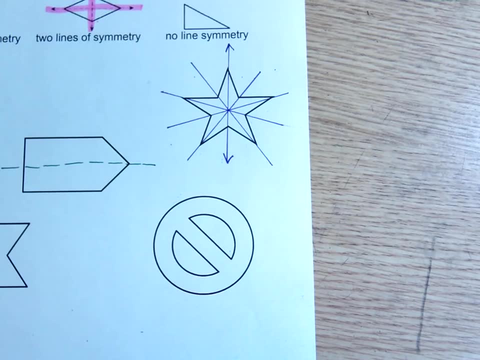 This is the bottom of the first one, so then that's the same line, All right. Next we have this band symbol, Not B-A-N-D, B-A-N-N-E-D. Okay, like if I'm going to ban you from doing something. 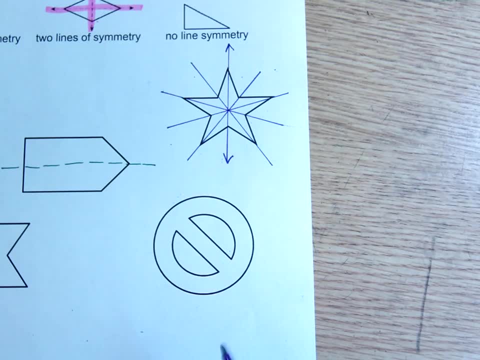 Or I could ban ghosts because this looks like the Ghostbusters symbol. Okay, So this looks like it has at least one line of symmetry. How many can you think of? I'm going to say there are two. I see a line of symmetry right down through the middle here. 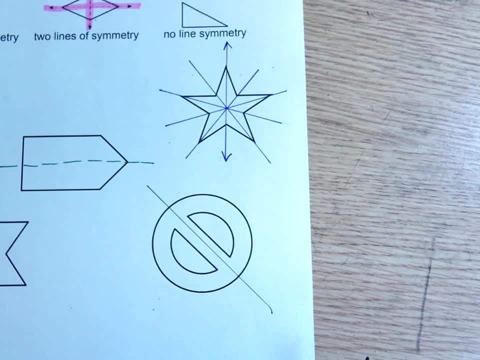 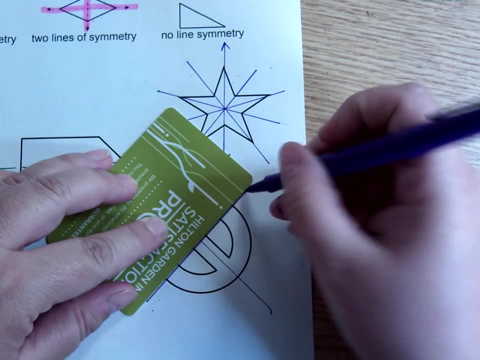 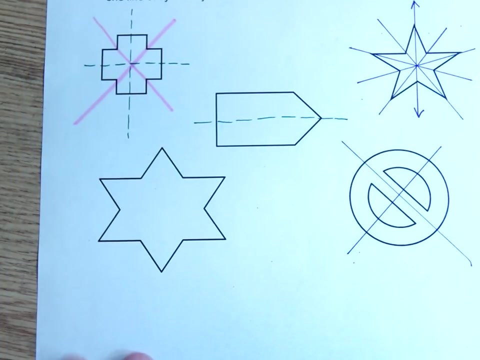 Like this, And I also see one going perpendicular to that. So I think I have two lines of symmetry there. Last but not least, I've got a Star of David over here, Or you could think of it as two triangles on top of each other. 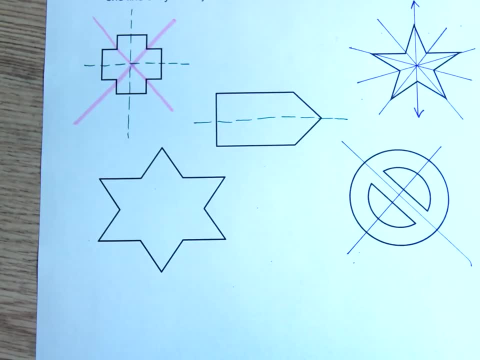 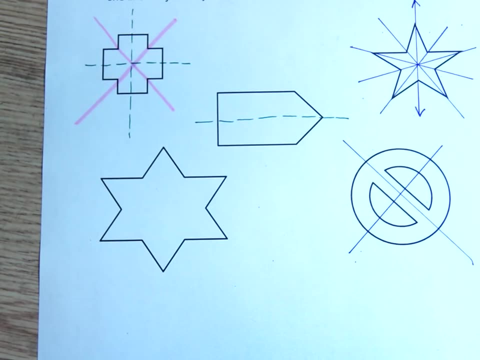 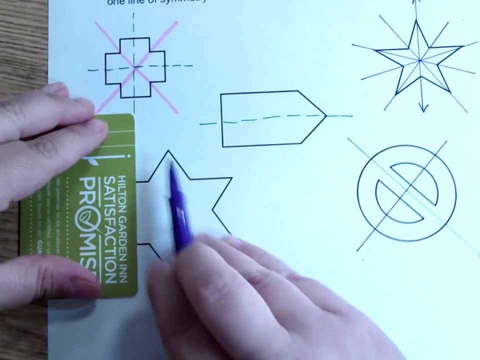 All right, This is full of symmetry. this one is, Again, assuming it's perfect. This one looks a little bit vertically squished, but pretend it's not. Pretend that this is a nicely symmetrical Star of David And we've got basically through any point of the star and the point across from it. 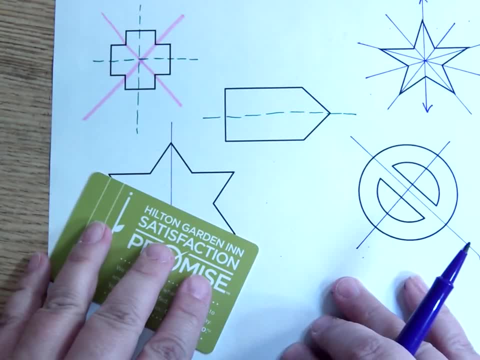 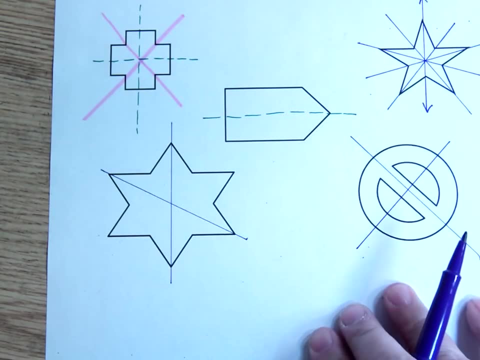 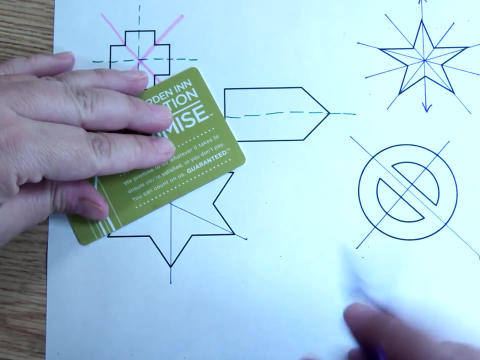 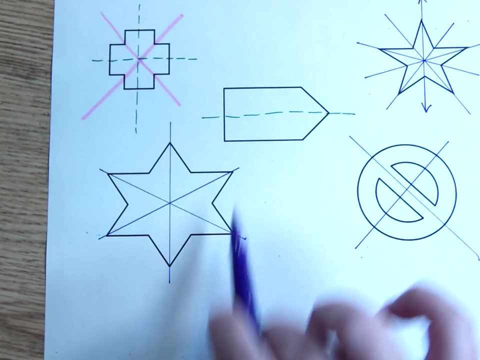 There we have it. Yeah, it is a little bit lopsided because this side doesn't look perfect, but But we're good at using our imaginations here, right? Okay, so each tip, each of the six points on this six-pointed star. 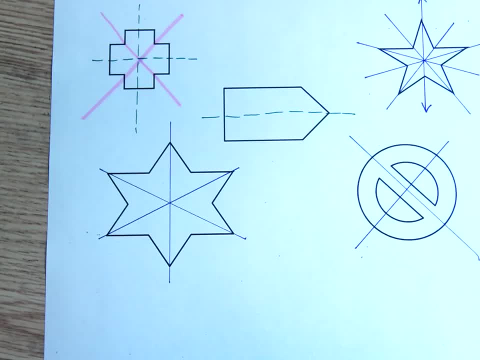 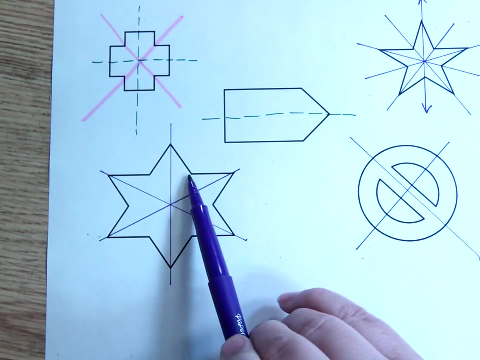 We can go straight through that line and go through the tip across from it. We could also go across or around this star, making lines of symmetry, if I can find my words- right through kind of the valleys in between the tips, In other words, this and the one across from it. 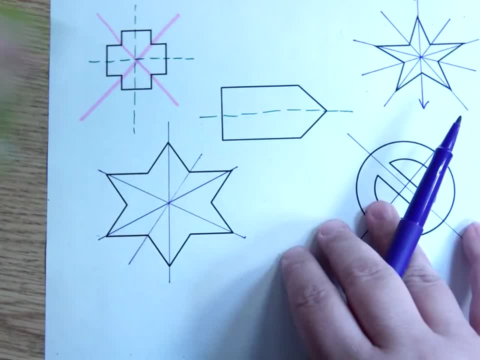 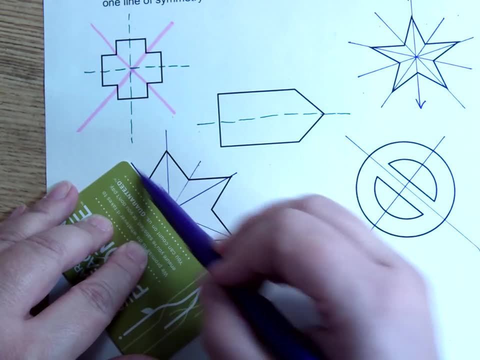 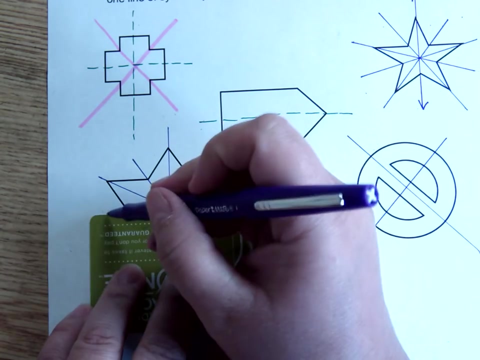 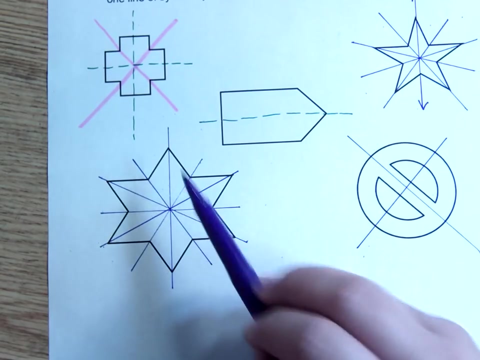 Right down through there and down through here and across here. So I've got symmetry all over the place in that. How many lines is that? Well, I've got one, two, three, four, five, six. Notice that on a five-pointed star I had five. 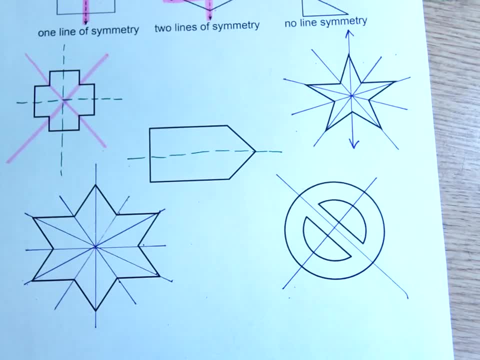 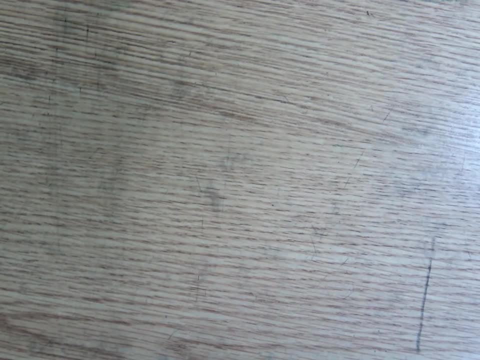 And on a six-pointed star I have six. So that's line symmetry. Now, another type of symmetry that we get a little bit more interested in now is rotational symmetry. So again, I made up a little blurb about it. 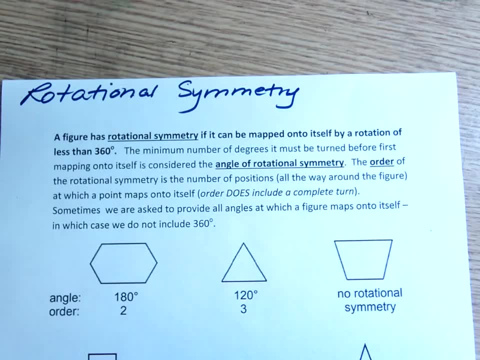 And I said, a figure has rotational symmetry if it can be mapped onto itself by a rotation of less than 360 degrees. Basically, if I want to turn anything in the entire world all the way around, it looks the same as it did before I turned it. theoretically. 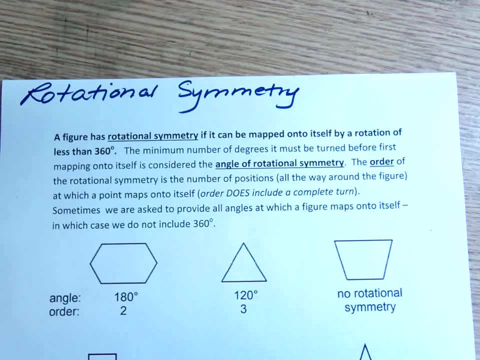 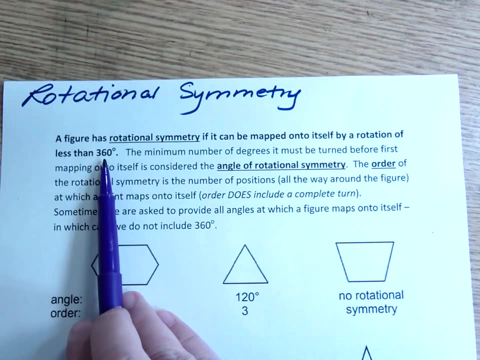 I guess something It could happen during that turn. But the point is the fact that it looks the same when I turn it. 360 doesn't have any meaning We're interested in. does it ever look the same when you turn it? less than a full turnaround? 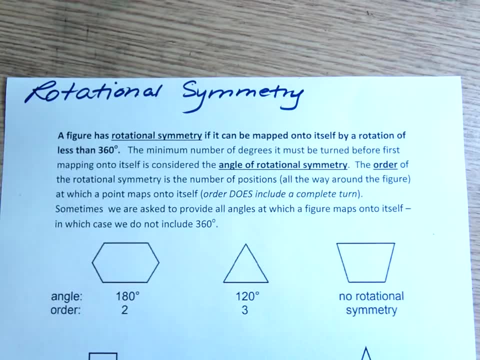 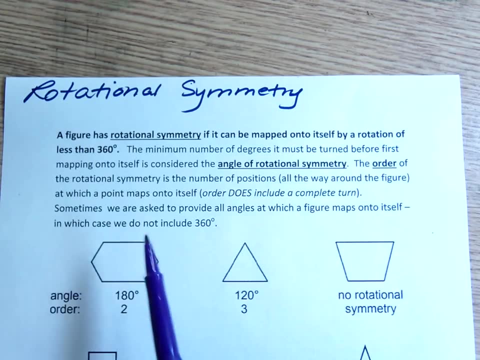 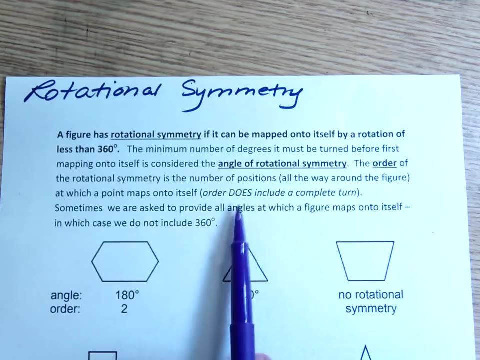 The minimum number of degrees it must be turned before first mapping onto itself is considered the angle of rotational symmetry. The order of the rotational symmetry is the number of positions all the way around, the figure at which a point maps onto itself. When we talk about order, we do include 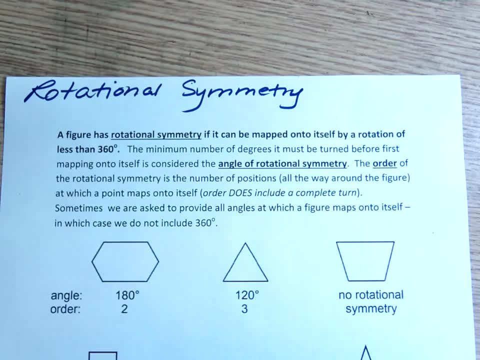 What if it's all the way around? Okay, so we do include that starting point as one of our points of symmetry. Sometimes we are asked to provide all angles at which a figure maps onto itself, in which case we do not include 360.. 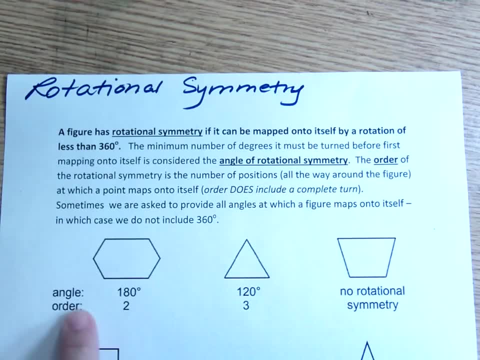 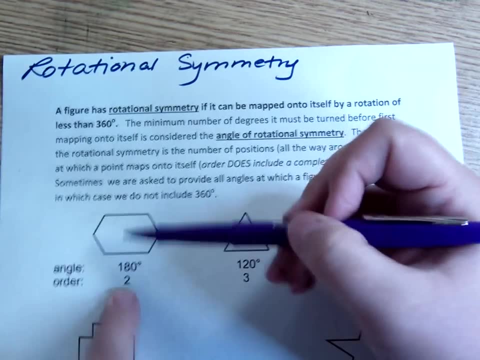 Okay, so here, looking at this, it says the angle is 180 and the order is 2.. So this is clearly meant to look squished vertically, so to speak. It's wider this way than it is this way, So it's not just a printing issue. 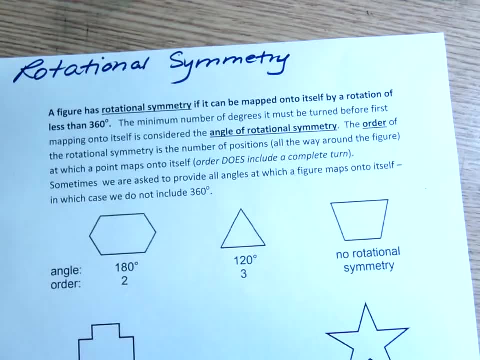 That's what it's supposed to look like. So if I took that figure and I flipped it completely upside down, that's what 180 means- I did a rotation of 180. It would look the same. So I'm going to use transparency to demonstrate that. 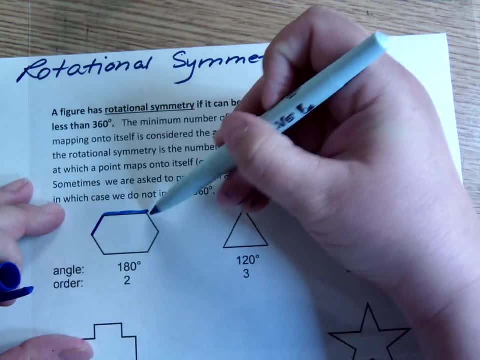 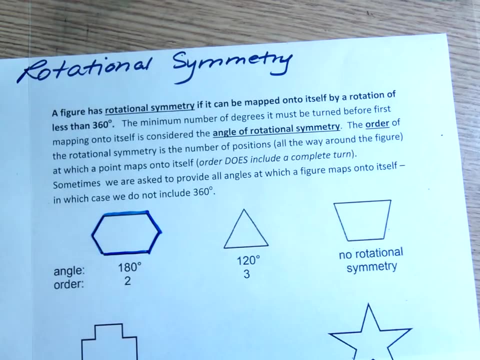 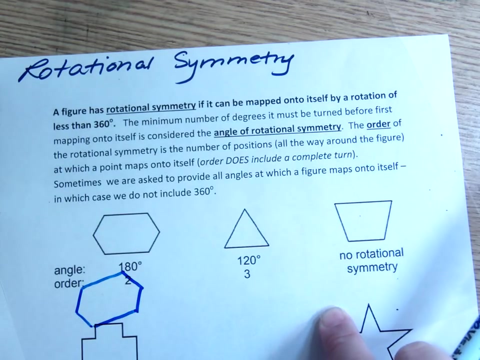 Trace it. And again, we're not going for perfection here, We're going for big idea. If I take that and I rotate it, and where am I rotating it? Well, if I rotated it like around, If I rotated it like around this point, then no, it's going, it's leaving, it's not going to map up onto itself. if I do that, 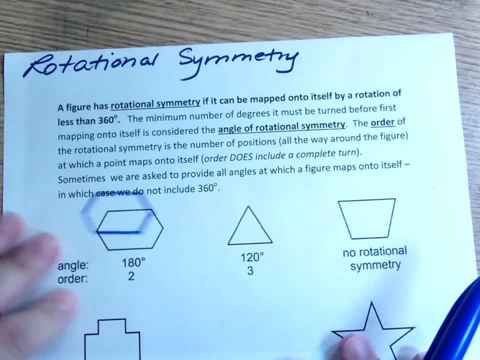 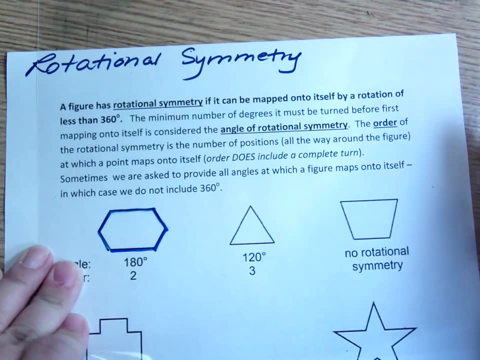 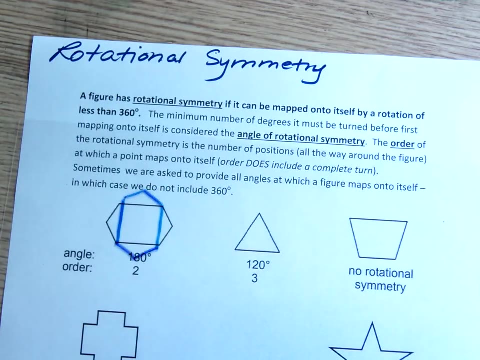 So we're not talking about that. We're talking about rotating it, about its own center, Rotating it in place, Okay, And I'm talking about like this: If I could hold that still, Alright, So this is 180.. Sometimes it helps to keep track. 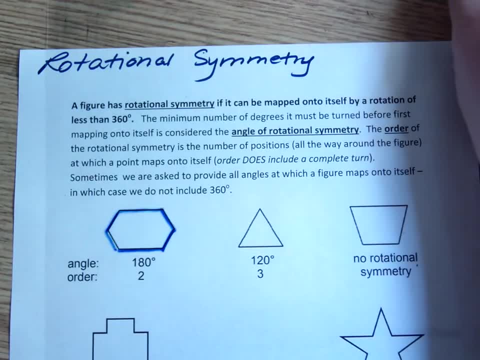 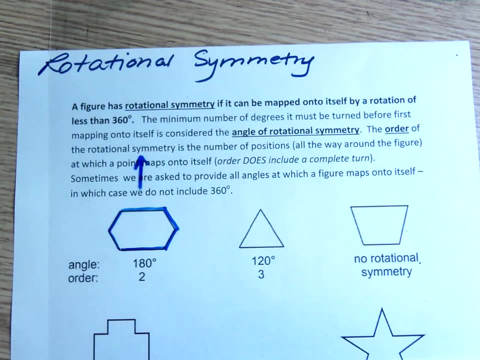 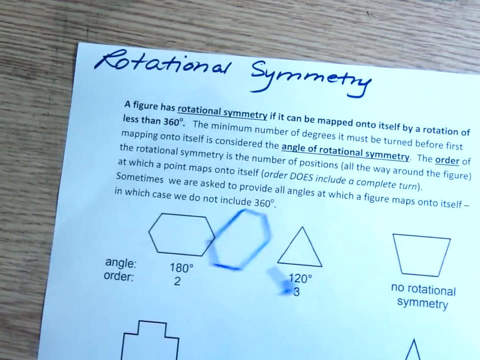 Let me put it back. Sometimes it helps to keep track of where you started by giving yourself a little reference: Okay, This is up. So after I spin it all the way around to where that's pointing downward, it matches. That's the first mapping. 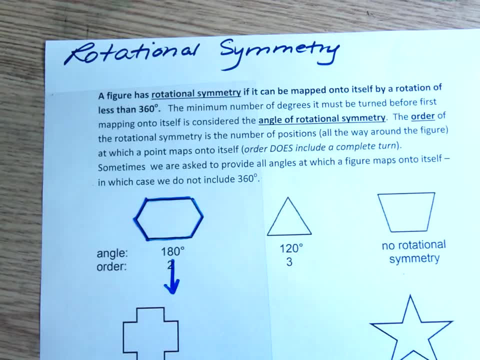 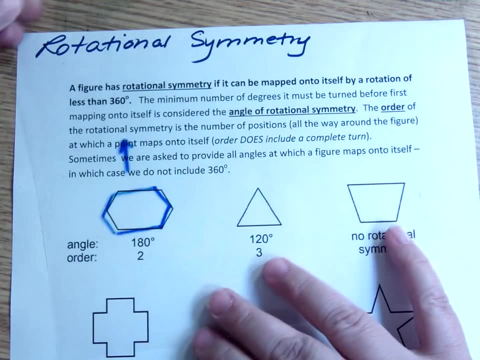 So that's 180 degrees, Because I've gone from the air pointing up to the air pointing down And, yes, when I turn it all the way around, it matches again. But that's not really rotational symmetry, That's just life. 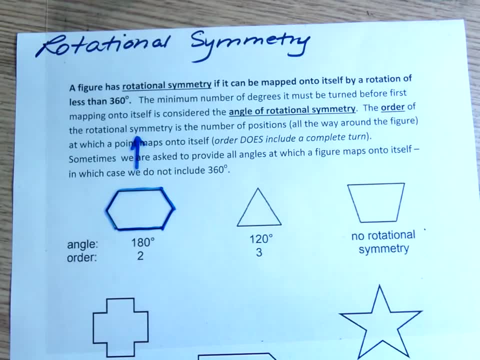 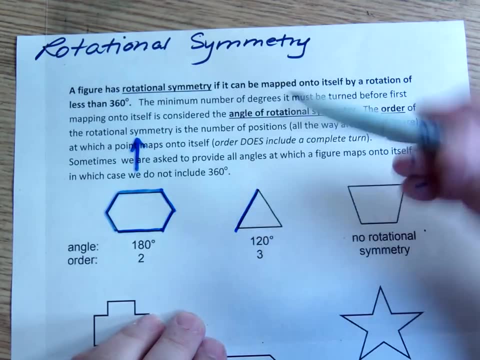 That's just what happens when you turn something all the way around. Okay, So let's look at this triangle beside it. Equilateral triangle is what it looks like, And I didn't. let me address this real quick. 180, we talked about. 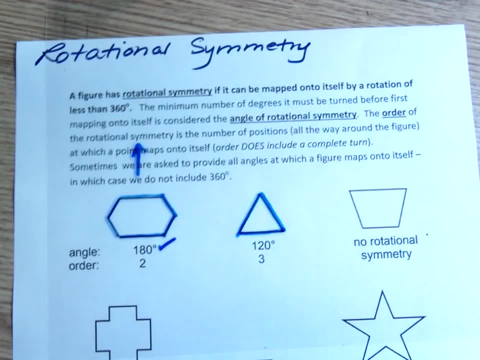 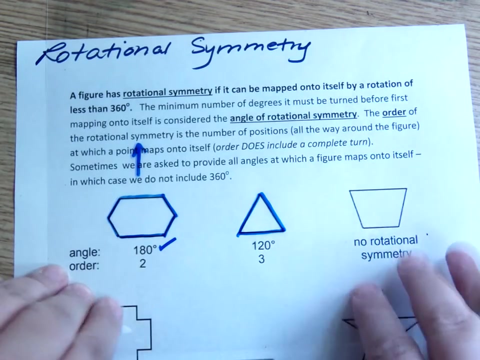 Two. the order of two basically means there are two positions. if I go all the way around, including starting place or the ending place, I don't want to count it both times, But there are two positions: that at which it looks the same, like this and exactly upside. 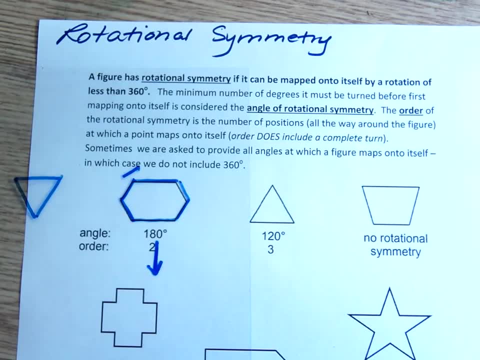 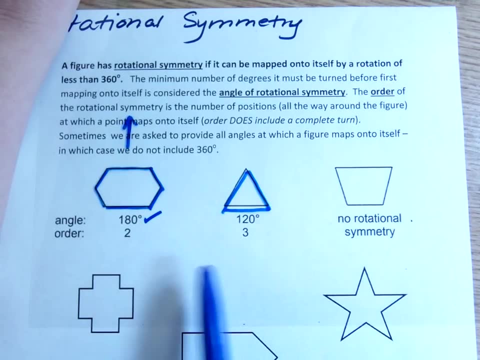 down like this: So that's why it's called a rotational symmetry of an order of two. Okay, So let's look at this triangle. It says that we have rotational symmetry with an order of three here, So that means we're talking about: there are three positions at which it looks exactly. 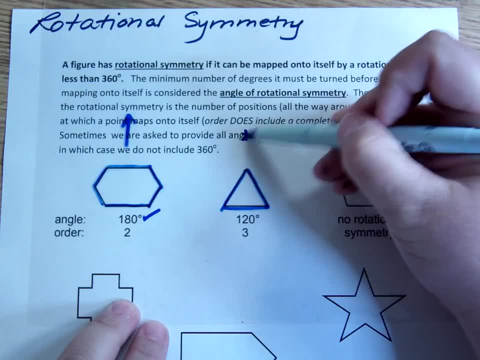 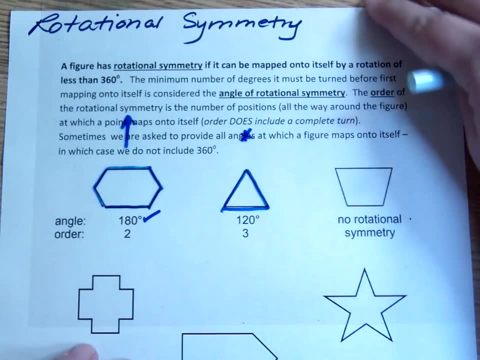 the same. So let's go ahead and make a little asterisk to point out: okay, this is what it looks like when it's straight up, Or this is with the asterisk up above the triangle. If I turn it, pretty much a third of the way around it matches up. 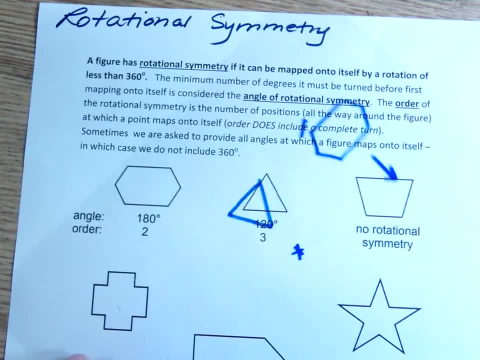 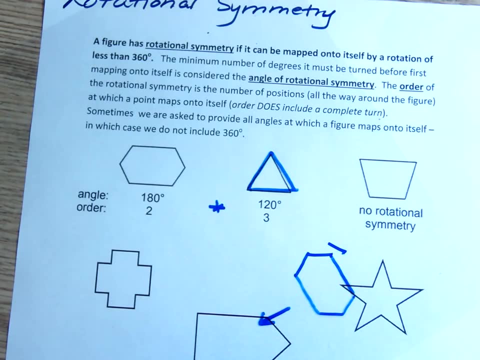 That's the second place it looks the same And if I turn it another third of the way around, which is two thirds of the way around, it matches up again. So that's the three places that it looks like. exactly the same figure as we rotate. 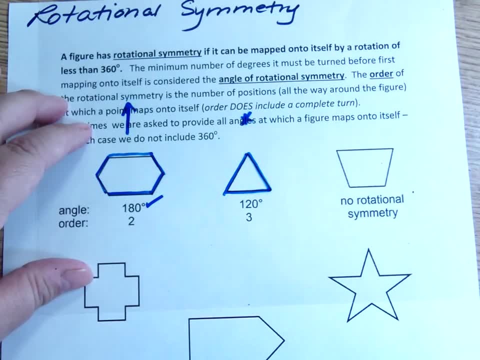 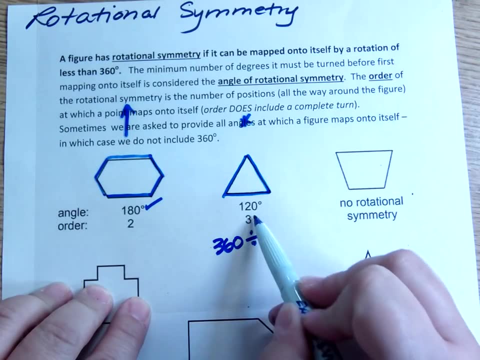 This is back to the first one I counted. Notice that if I divide 360 by this number- the order- what do I get? I get 120, which is exactly what this says. It says that after I've rotated at 120, that's when I get to the first point at which it 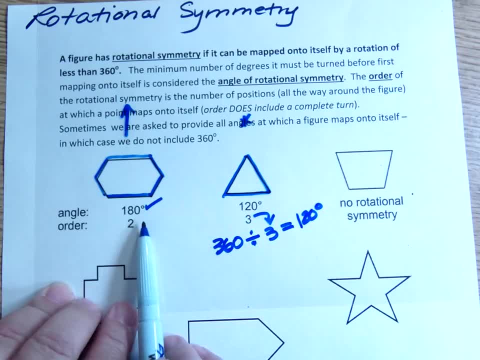 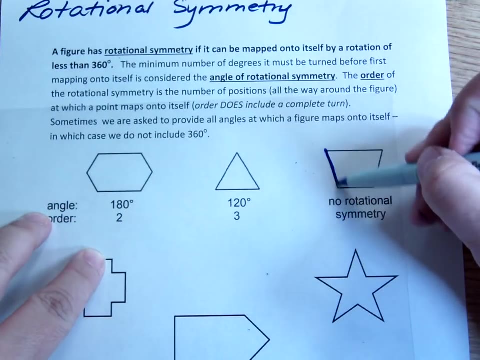 matches up Same thing over here. If my order is two, then my angle of rotational symmetry is 180, because 360 divided by two is 180.. Okay, So this one has no rotational symmetry. Let me give it some space here. 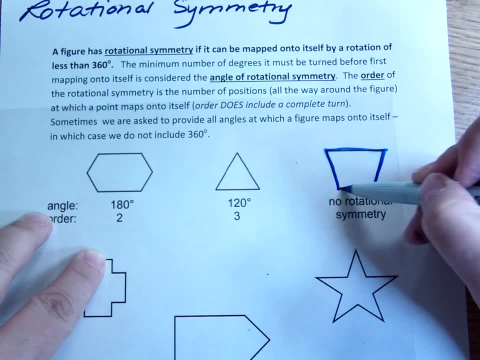 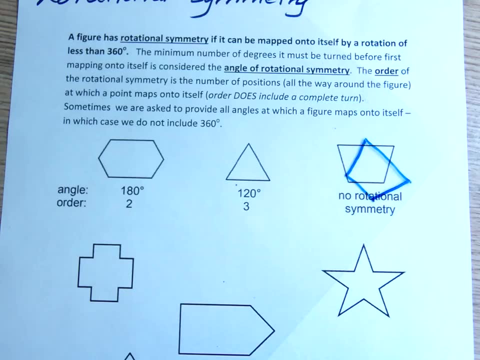 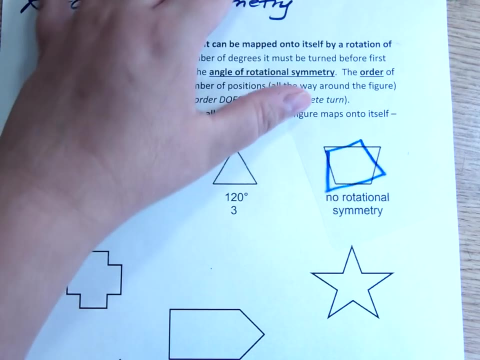 Okay, If I rotate this around on top of itself, nowhere does it map up, It doesn't look right, It doesn't get right on top of itself. So sorry, This is not the most accurate way to do this. Sorry, I think you can get the idea pretty well though. 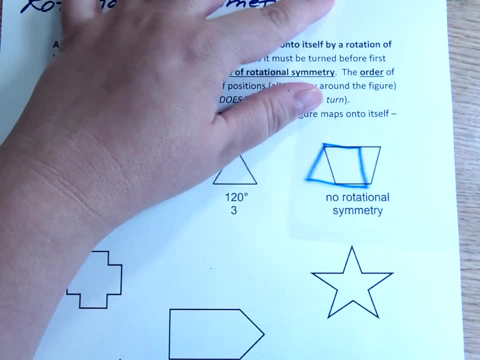 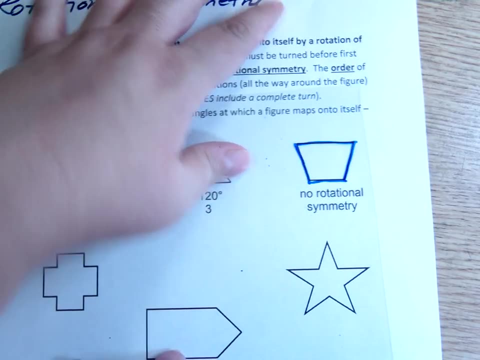 Here is a 180.. Notice it's not matching up. Okay, Okay, Okay, Okay, Okay. Nowhere does it match up until you get all the way back around, which, like I said, that doesn't really count as having rotational symmetry. 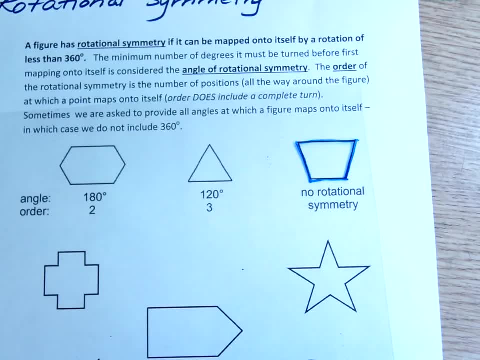 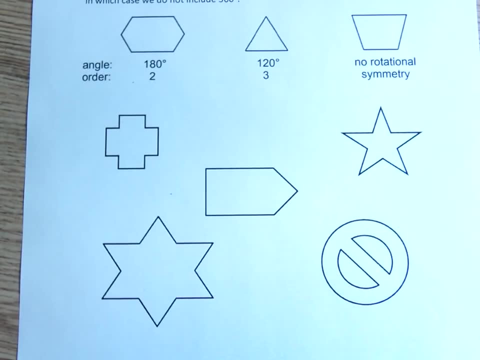 Okay, So let's look at these same figures we used for the line symmetry. all right, This one that looks like a red cross arrow: How many places all the way around does it look like it would look the same? Let's try. 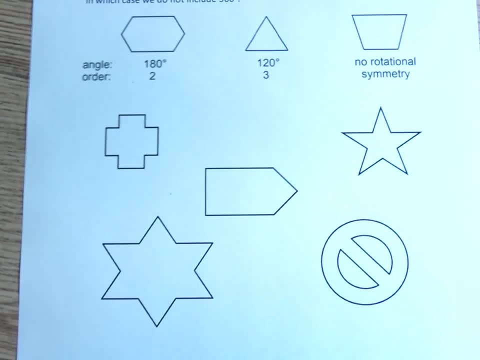 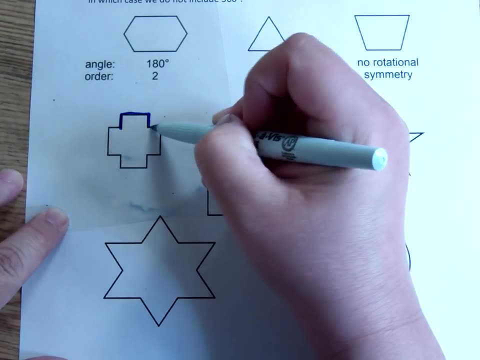 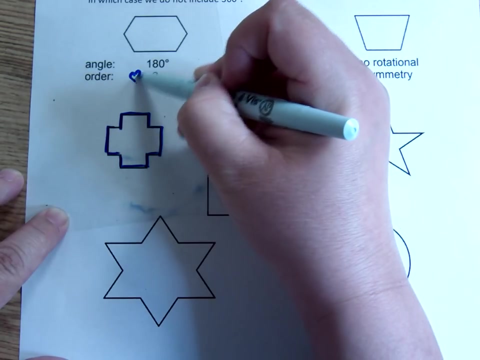 Let's try Now. I'm going to put something on the top. I've used an arrow and a little asterisk- It's a little heart this time- just to remind me that that's where I was when I started. Okay, 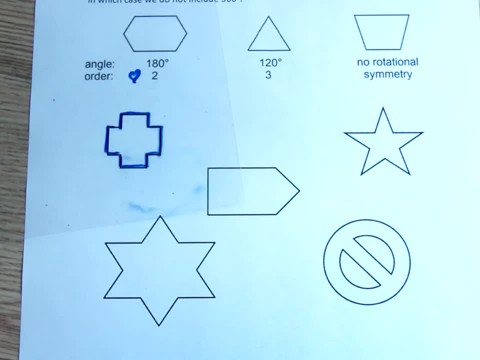 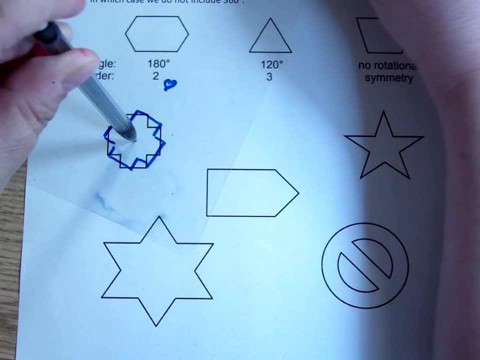 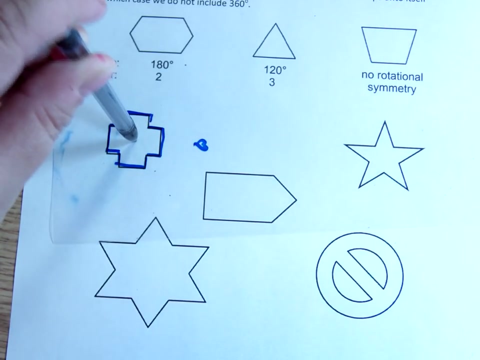 Let's see if I can spin this a little bit more effectively or efficiently using a pen or, excuse me, a pencil as my center. There we go. Okay, that's my center of rotation. If I turn it so that the heart is at the side, it matches up Well. if the heart started at the top and then 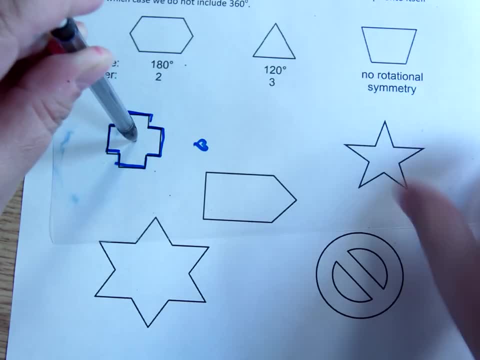 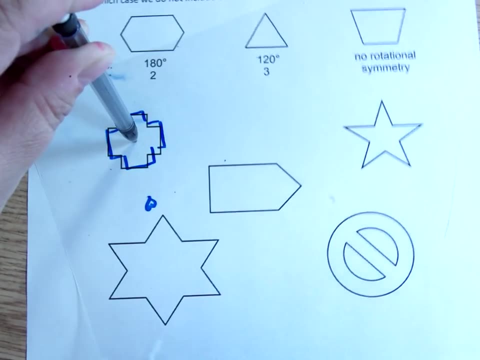 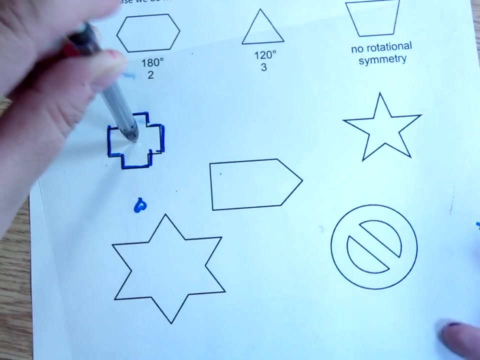 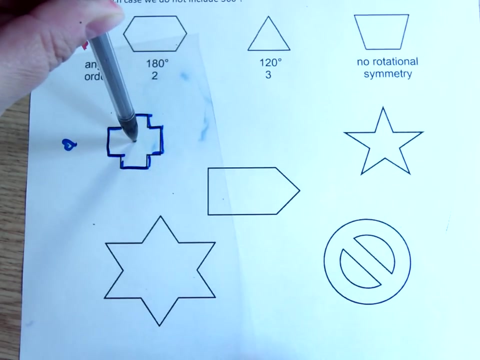 now the heart's at the side. I've rotated it 90 degrees, So after 90 degrees it matches up, And again when the heart is at the bottom. that means I've gone 180 now And it's also going to match up. I can get out of the way of the camera at 270.. And then we get back. 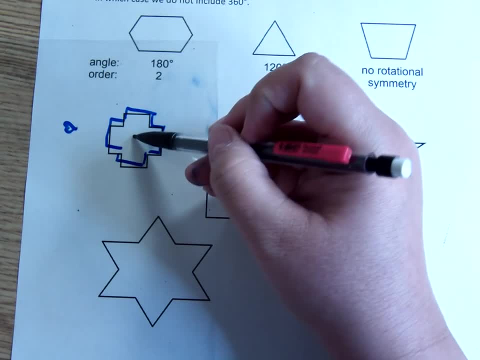 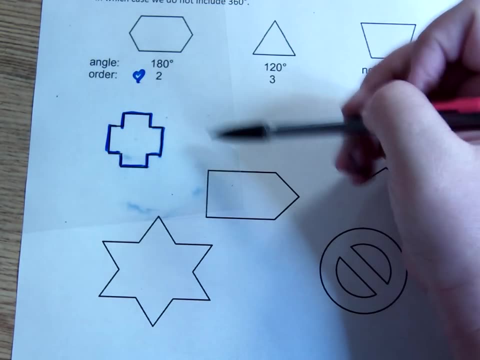 to our starting place. Okay, So including the start, and then we're going to get back to our starting place. When the heart was here, the heart was here and the heart was here. there were four places at which it looks exactly the same. 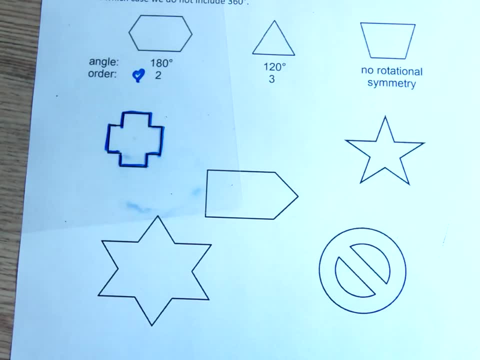 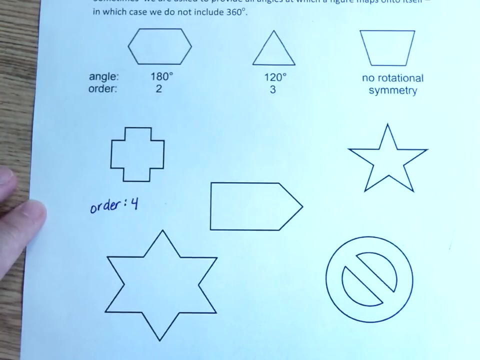 Not counting the heart, because the heart's not really part of the shape anyway. So that has an order of four. okay, Now, if it has an order of four, what's the minimum angle? Well, we set up above here that if I divide 360 all the way around, by the order I find, 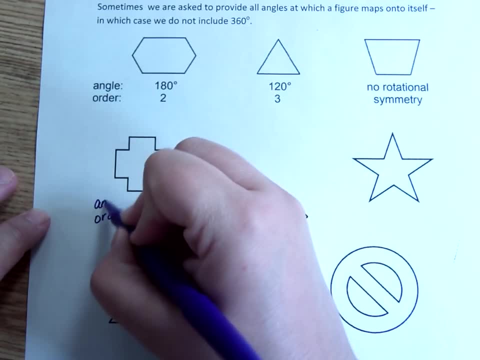 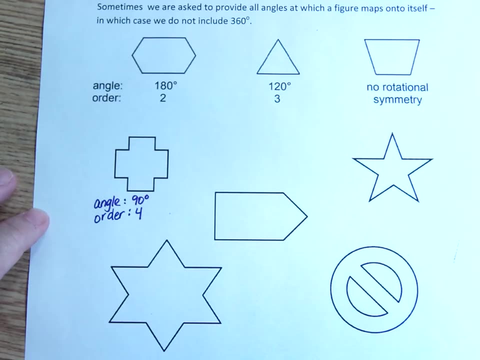 out what the angle of rotational symmetry is, and that's 90 degrees. Every time I turn it 90 degrees it'll match up again. Sometimes, the way this is asked and this is up here- it says this: sometimes it'll say: 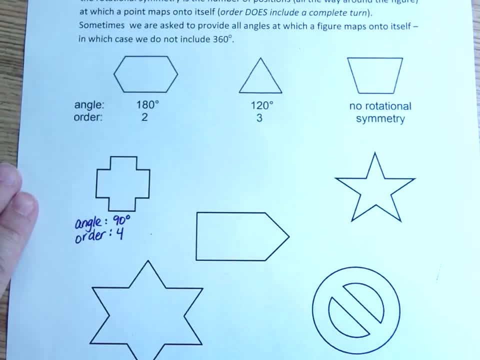 name all angles at which the figure maps onto itself. Well then, I would say 90,, 180,, 270.. I'm not going to list 360 or 0, because that's the starting place and we know that we're back at the starting place at 360.. 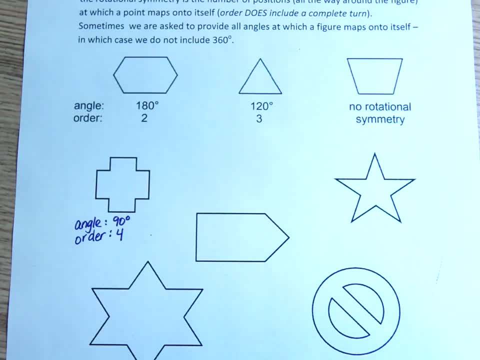 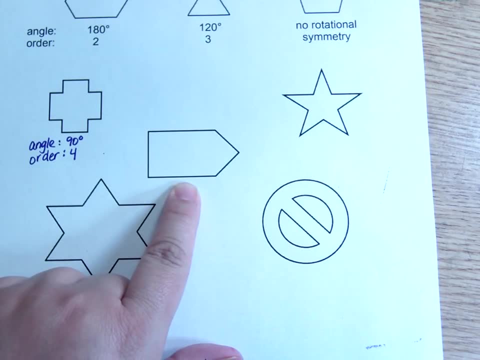 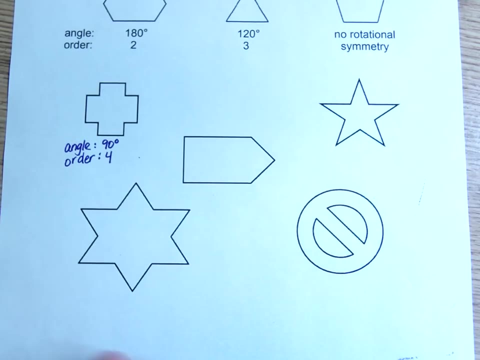 So we're talking about angles, Really between 0 and 360.. That's what we're interested in. Okay, let's look at this figure. This figure has no rotational symmetry at all because it's pointing to the right now If I start turning it- and I think this time I'm just going to turn the paper if I start- 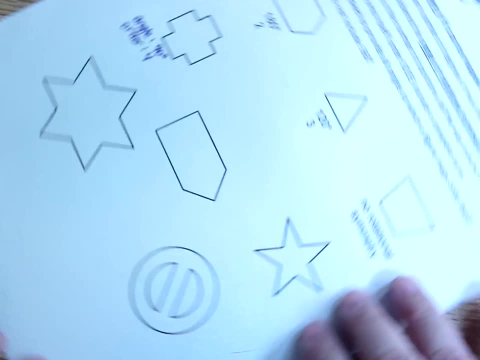 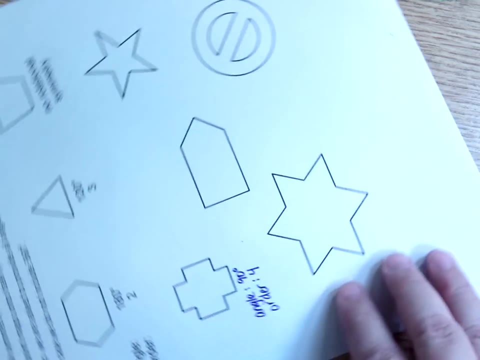 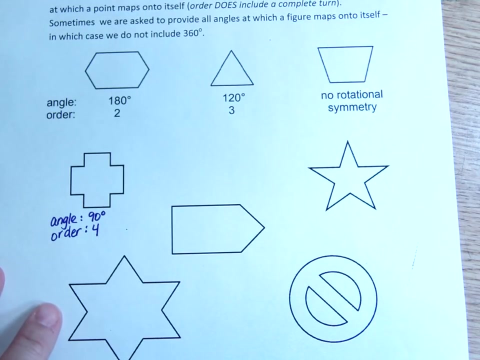 turning it. now it's pointing down, now it's pointing to the left, now it's pointing up. It's not until I get all the way back around that it looks the same pointing to the right. So that's not rotational symmetry. 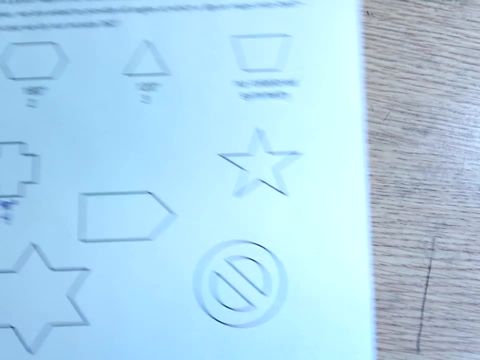 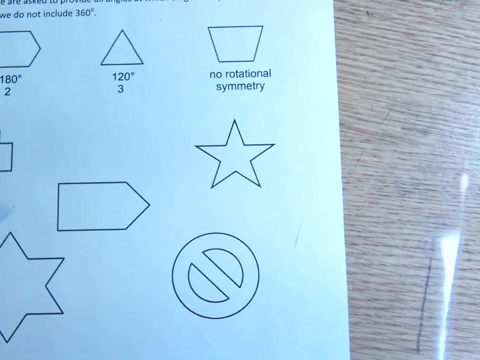 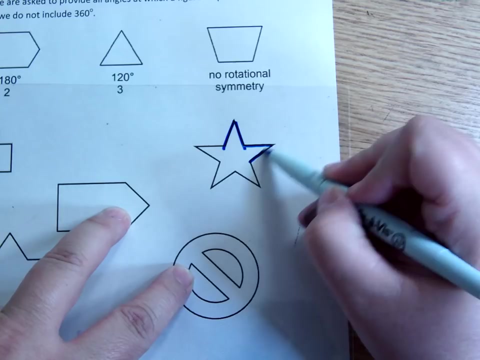 However, hopefully you noticed, as this star was rotating, it should look the same several different places. So let's look at the star. I'm going to trace the star on my transparency paper. I already went over the edge a little bit there. not the most accurate tracing. 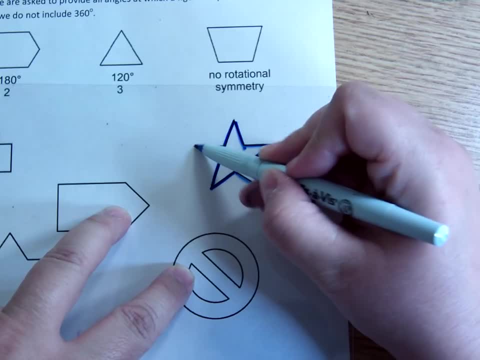 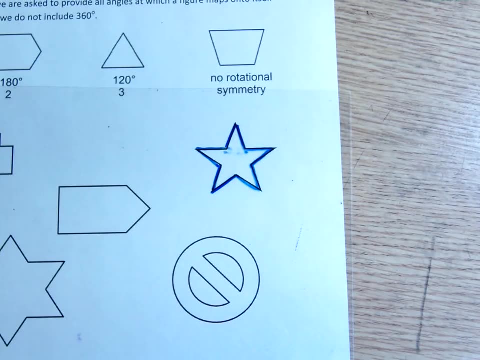 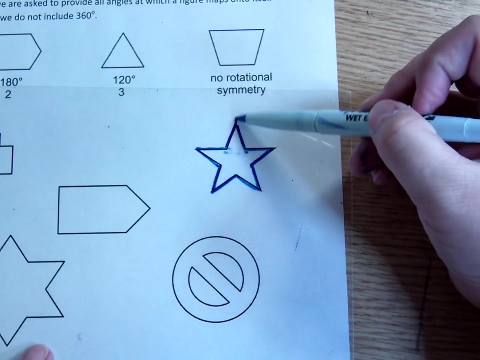 Okay, Okay, Okay, Okay, And I tried to fix it and I don't know that I did much, but that's okay, Alright. so let me make this a little bit taller than the other ones, just to point out this was where I started with that pointing up. 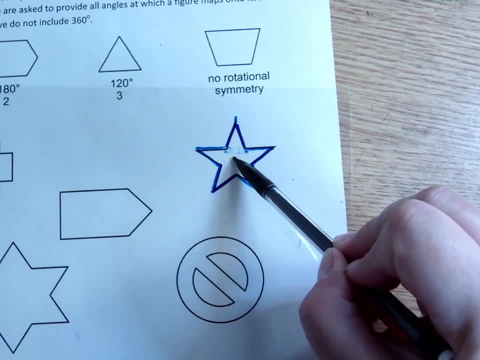 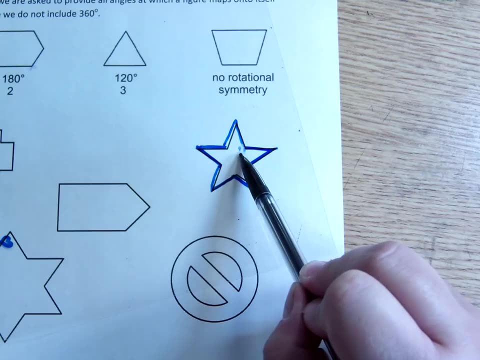 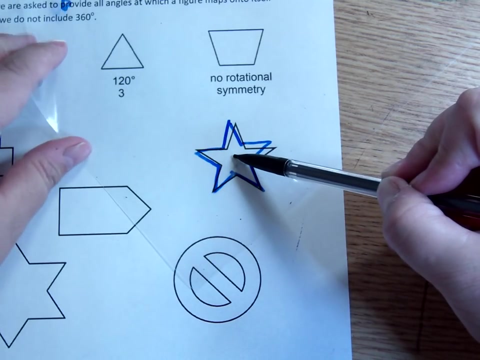 Okay, Now it looks fine there. Now just a little bit. I haven't even rotated that much and it matched up. I'm going to rotate again Here it matches up again. And rotate again. Here it matches up. How many times do you think? 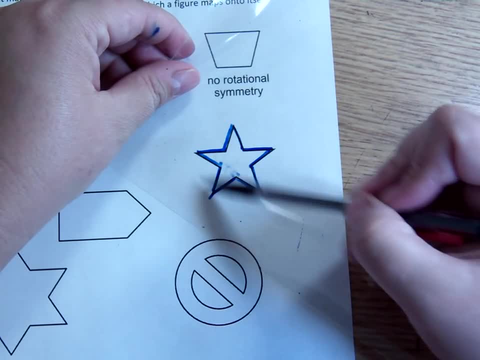 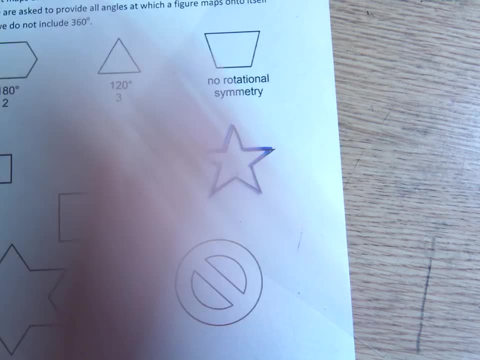 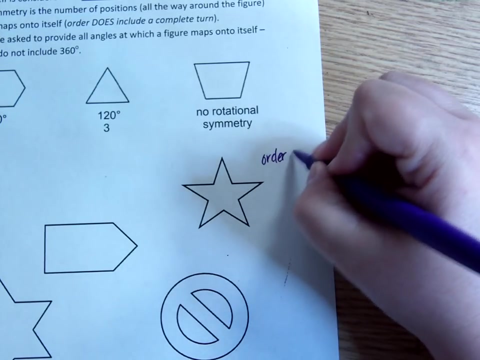 Well, look at how many points there are. There are five points. That's going to be five times. It matches up perfectly, And 360 degrees divided by five will tell me what each angle is. So here I've got a rotational symmetry of order 5.. 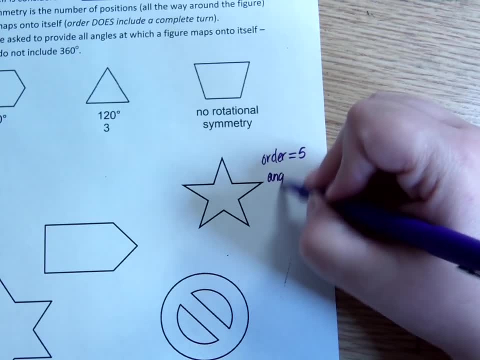 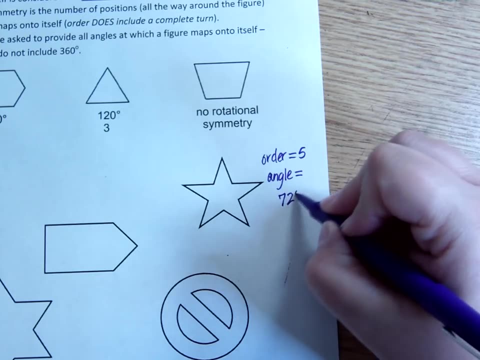 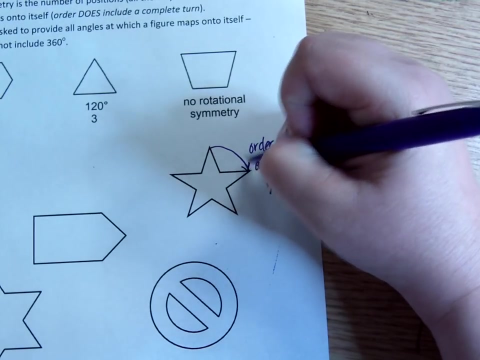 And the angle of rotational symmetry is 360 divided by 5.. 360 divided by 5 is 72 degrees. So every 72 degrees this will match back up. In other words, from here to here is a rotation of 72 degrees. So if you were asking me, 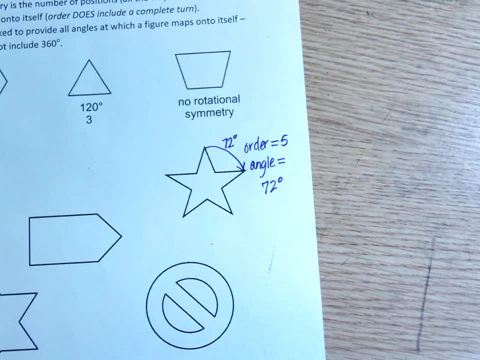 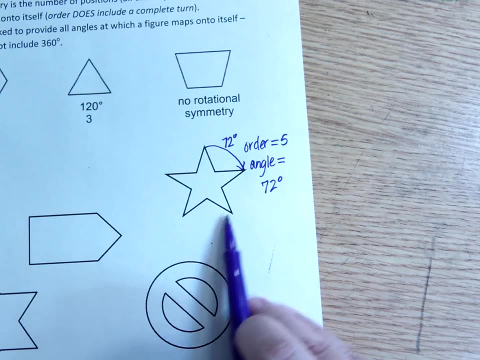 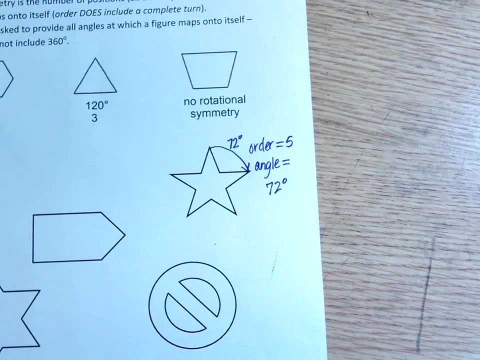 name all the angles at which it maps onto itself. I would say 72. And the next one would be 72 plus 72, which is 144.. And the next would be 216. And the next would be 288. And then we don't have to name 360, because 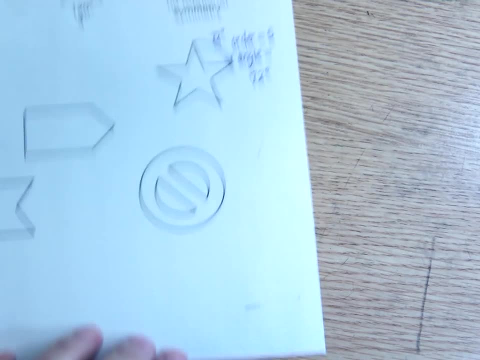 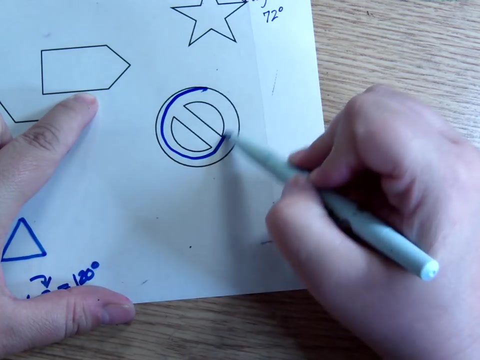 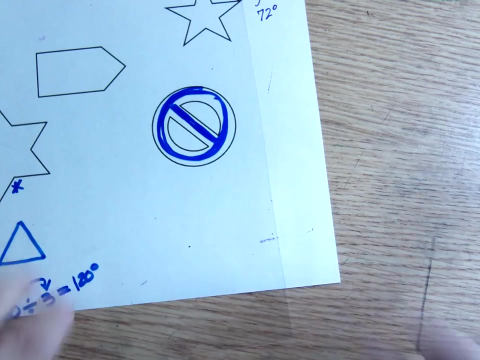 pretty much understood. Alright, let's go ahead, do our little Ghostbusters. BAM symbol, And I'm not gonna trace it that painstakingly, I'm just gonna draw big circle and a little slash mark, Okay, And see if I spin it about itself, about its own center. 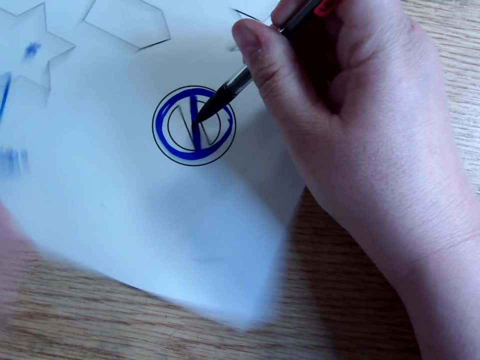 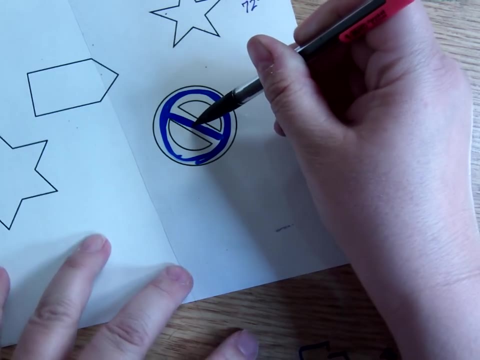 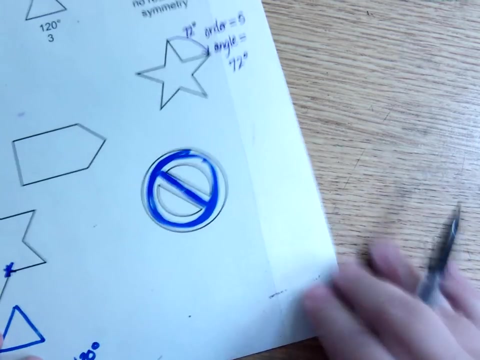 rotate it in place without taking this paper with it, if it ever matches up before it gets all the way back around. And yes, after 180 degrees. in other words, this let's go ahead and say this is up. 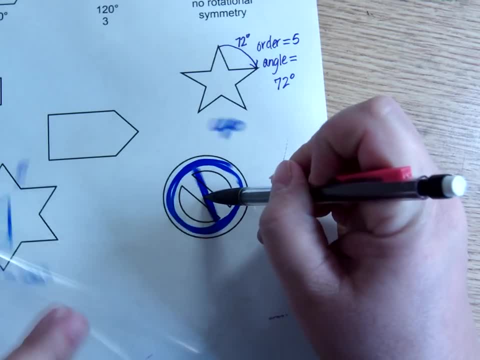 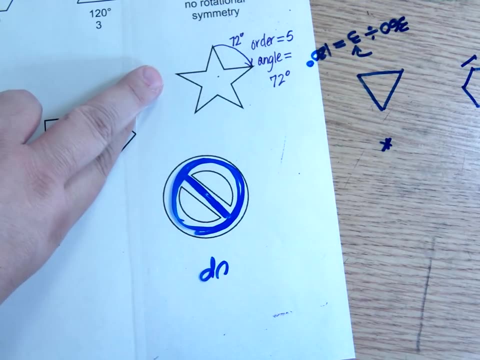 When I rotate it 180, so that up is down now it matches up, or it matches, not to use the word up in a different context. Okay, so that means that we have rotational order two. rotational symmetry of order two. 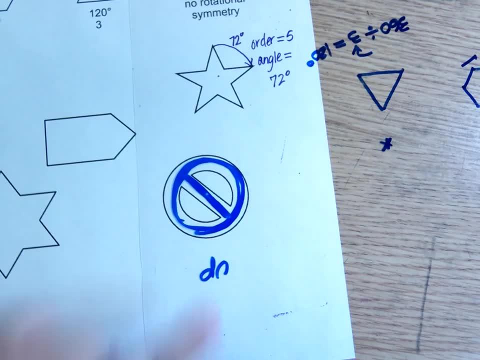 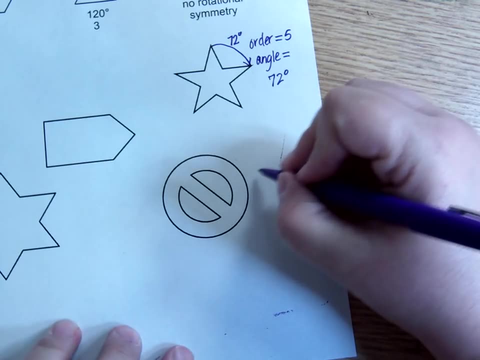 because there are two places: when this is pointing up and when this is pointing down that it looks the same. And 360 divided by two is 180.. So this has order two and 180 is my angle Angle of rotational symmetry. 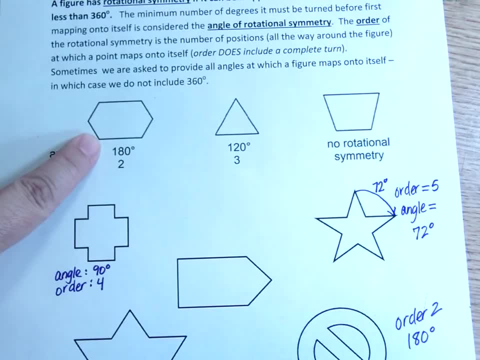 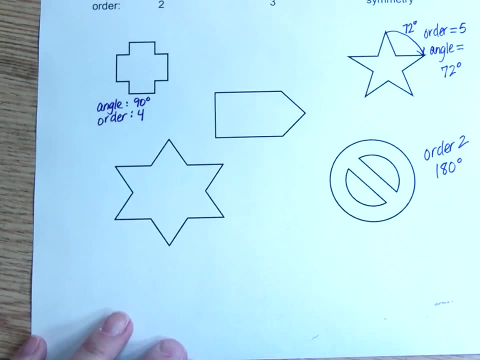 a lot like this one up here. Now this one should have a little bit more than the others because it had more lines of symmetry. So I've got a six pointed star here. I'm going to running out of space on my little transparency. 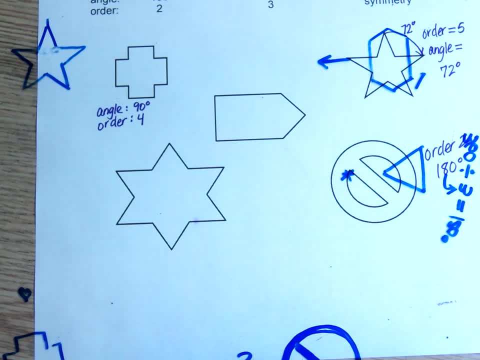 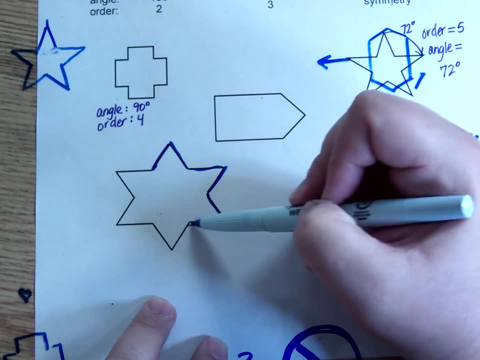 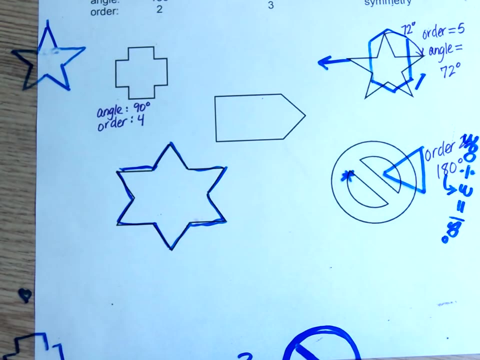 I'm using here. trace it Now. this star is, I believe, a little bit compressed vertically, So I don't know that it's gonna look perfect, But we're gonna pretend it's pretty symmetrical. Okay, so go on a journey of imagination with me. 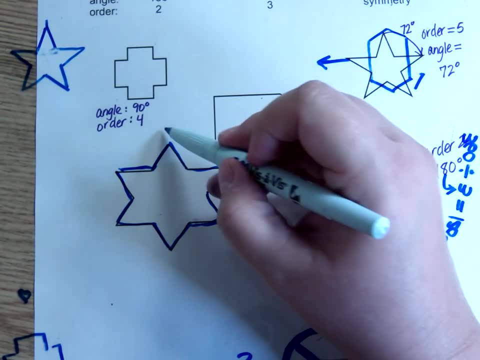 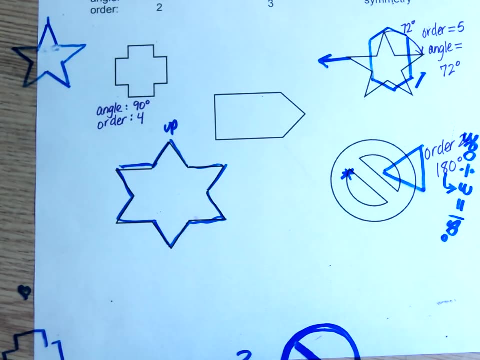 And let's say that this is up, How many times do you think it will match up to itself If I count the starting one as one? How many points are there on the star? Well, six pointed star, we should be able to find six places, six positions. 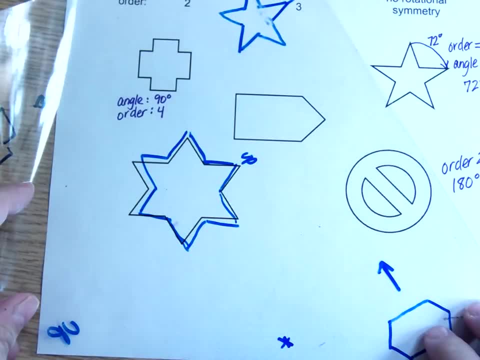 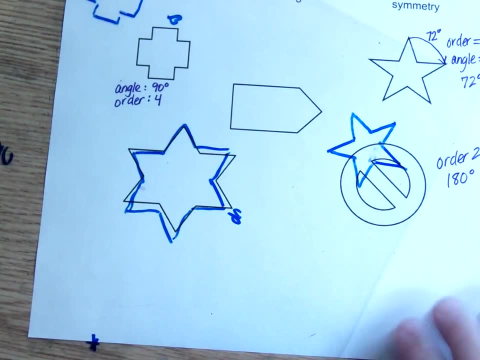 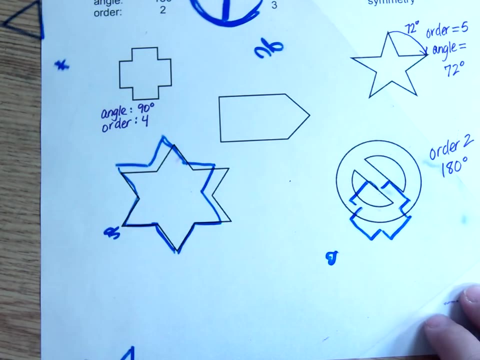 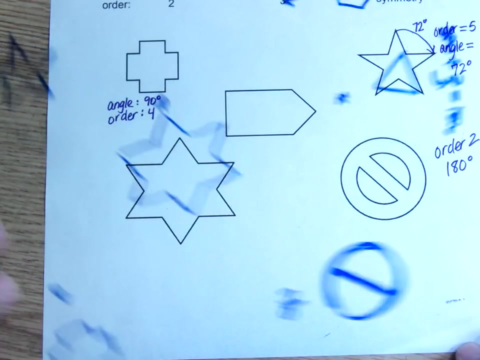 in which it looks the same. There's a second position. See how it's not quite, but you get the idea. Third position, Fourth position, Fifth position, Sixth position- And this was my first position, So you can kind of think of it as: 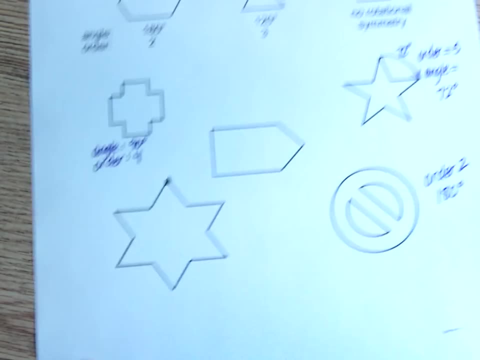 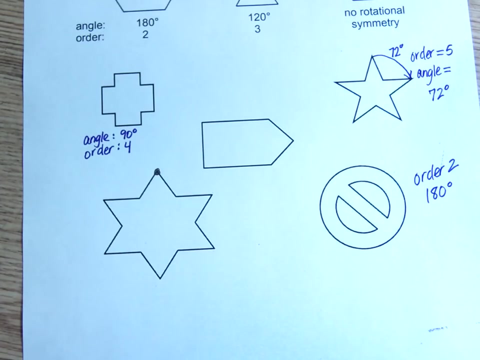 this point moves through these other points And each time it lands on top of another point we have an angle of rotational symmetry. So in other words, when it goes over here matches up again when it's on top of that, Then again when it comes over here. 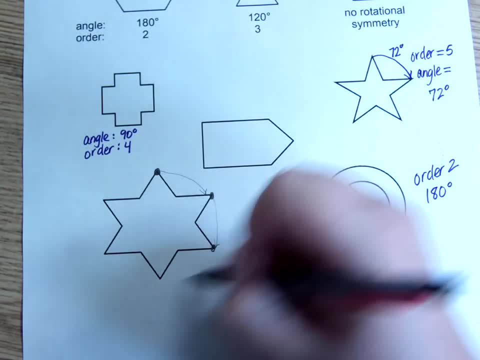 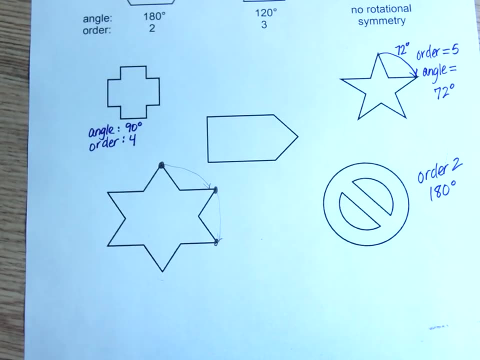 it matches up again and so on. So there's six times or six different ways I can turn this figure and it looks exactly the same. So that's order six And that means that I divide 360 divided by six to find my angle. 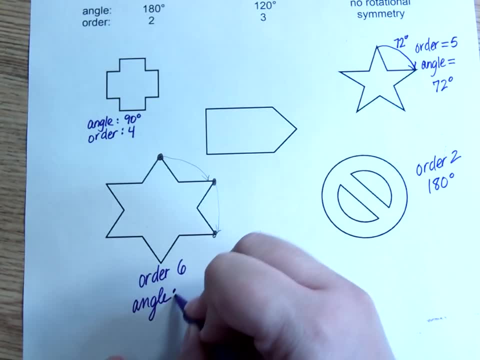 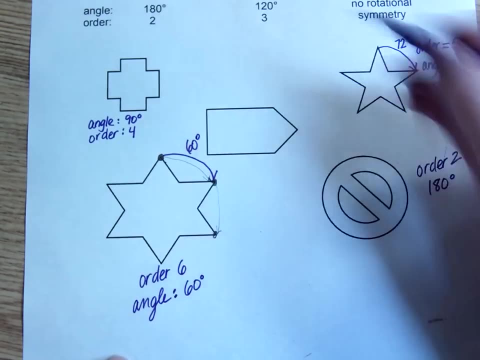 The angle of rotational symmetry is 60 degrees. So every 60 degrees that I turn it's going to match up again. So that means at 60 degrees, at 120 degrees, at 180,, at 240, and at 300. 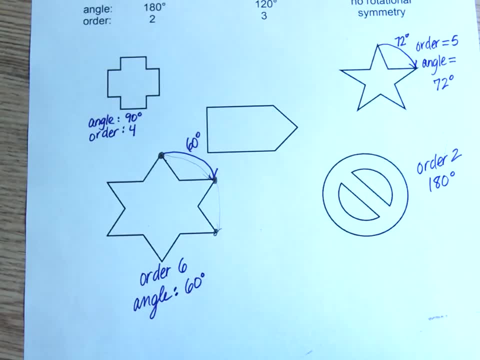 And that, my friends, is rotational symmetry in a nutshell. Hope you enjoyed it.